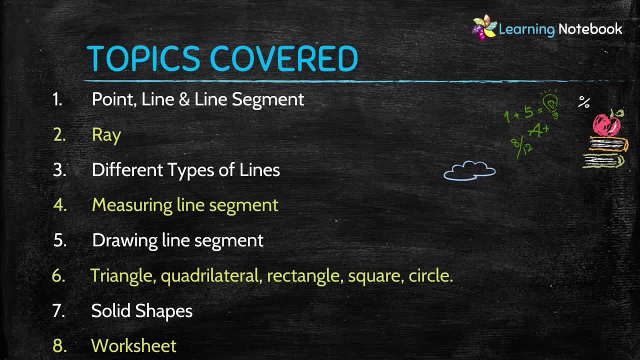 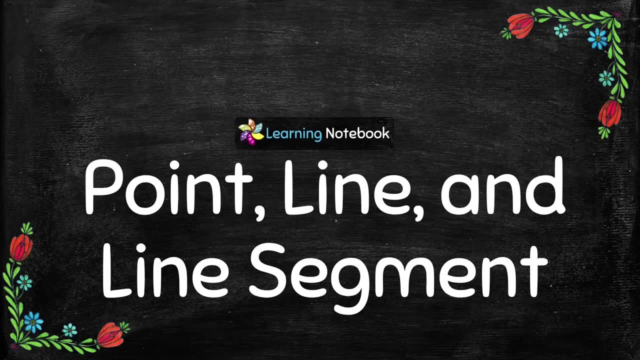 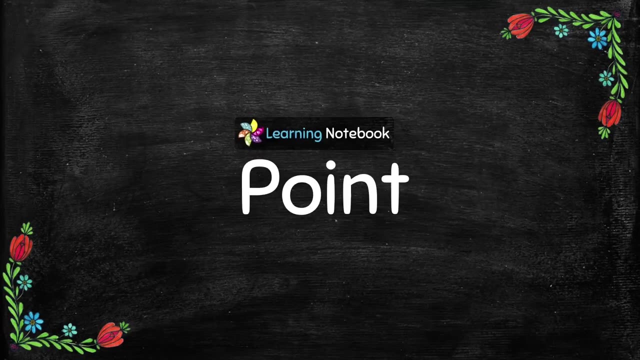 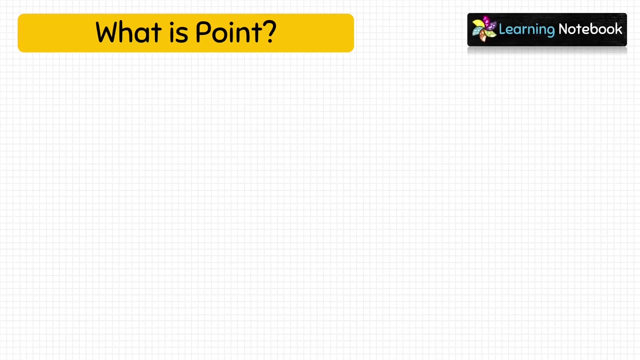 And in the end I will give you a worksheet on geometry for your practice. So let's start with our first topic: Point Line and Line Segment. First we will understand what is Point. Point is the basic unit of geometry. 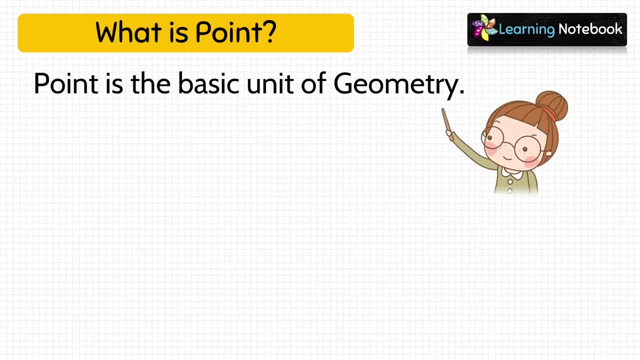 A point shows an exact location. It has no dimensions. That means a point has no length, breadth or height. A point is represented by a dot And it is named with a capital letter. For example, this is Point A, Point B and Point X. 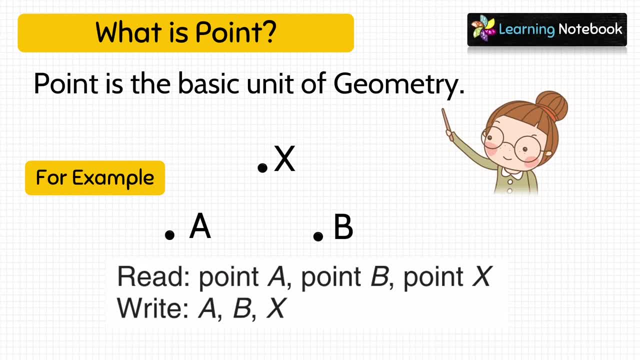 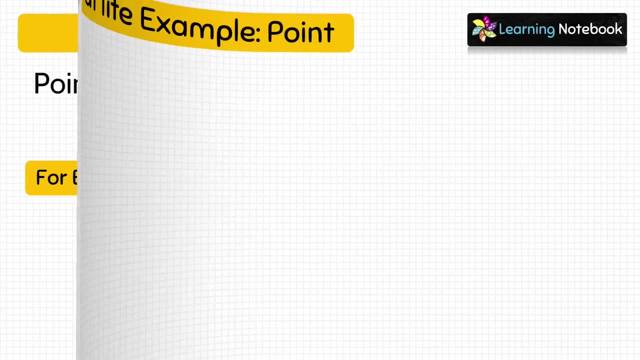 So how do we read this? As I just told you, we will read them as Point A, Point B and Point X. And how do we write these points? We will write them as A, B and X. Let me tell you a real-life example of a point. 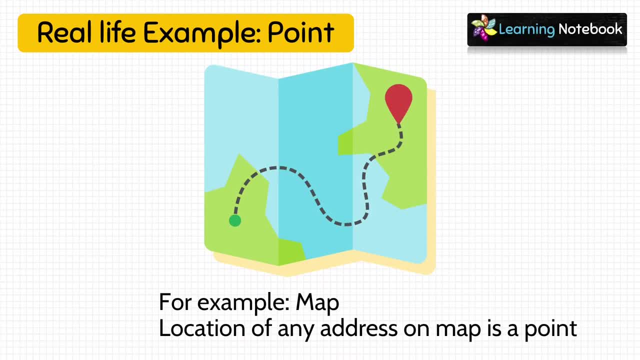 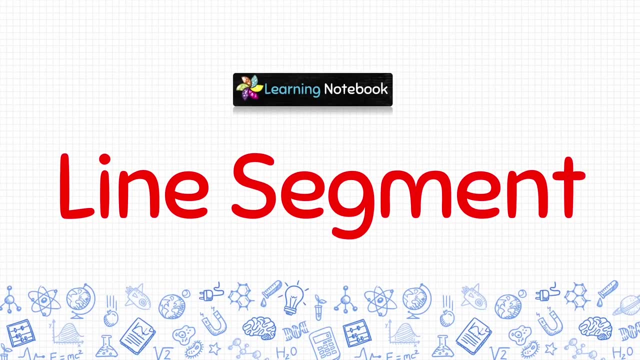 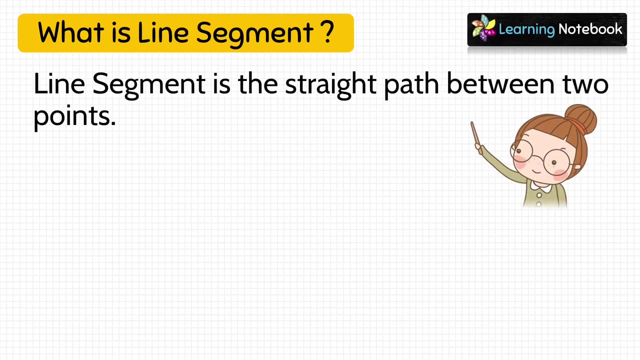 For example, location of any address on map is a Point. Next is Line Segment. A line segment is a straight path between two points. It is the shortest distance between two points. For example, there are two points DE, So line segment is the straight path between these two points. 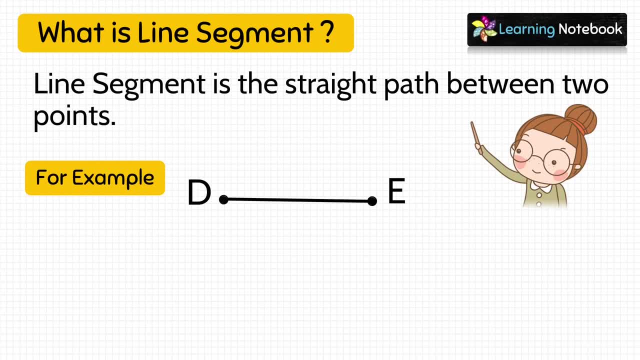 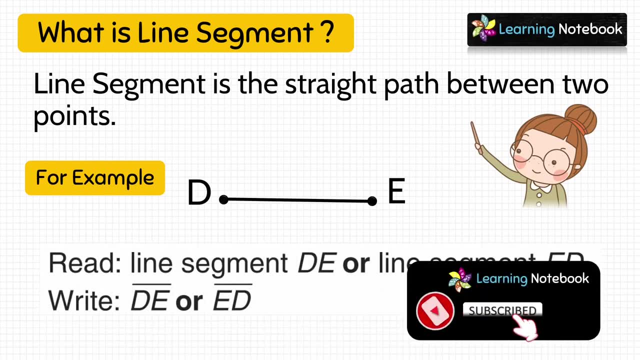 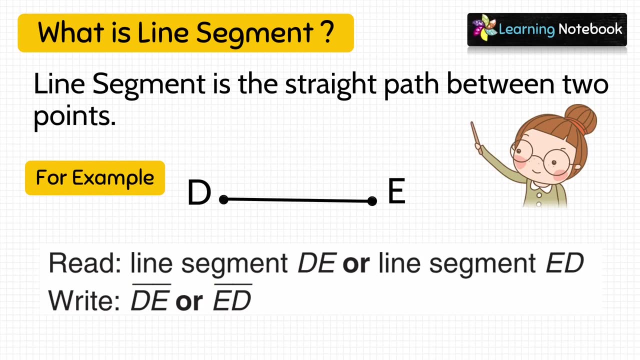 Now let me show you how to read and write line segment. We will read it as Line Segment DE or Line Segment ED. Both the ways are fine. Similarly, we can either write it as DE or ED with a small line segment on it. 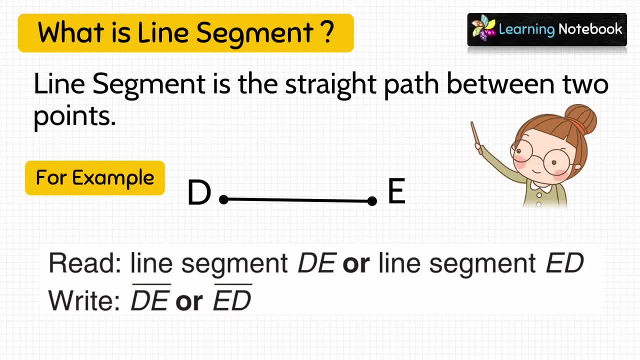 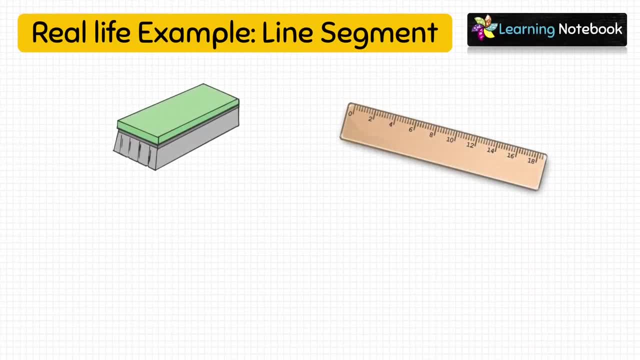 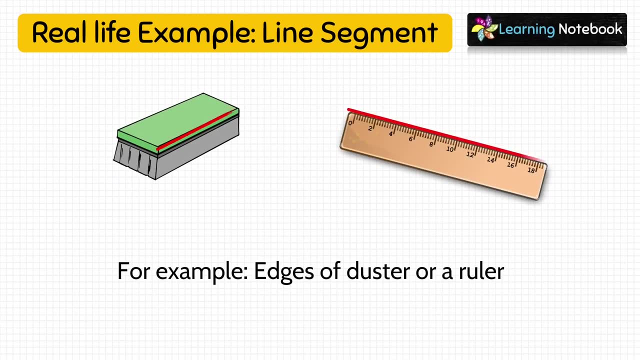 Also, students do remember that a line segment has a point. It has a definite length. Now let's see some real-life examples of line segment: Edges of duster or edges of a ruler. They are line segment because they have a definite length. 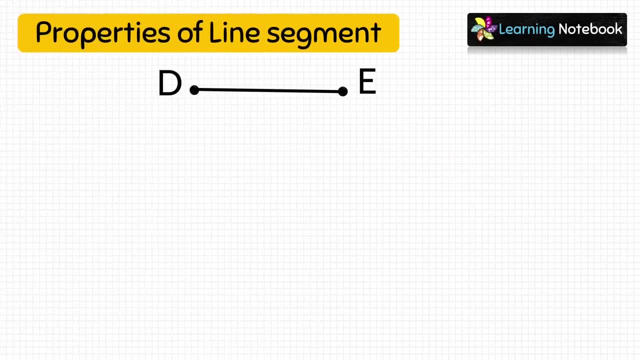 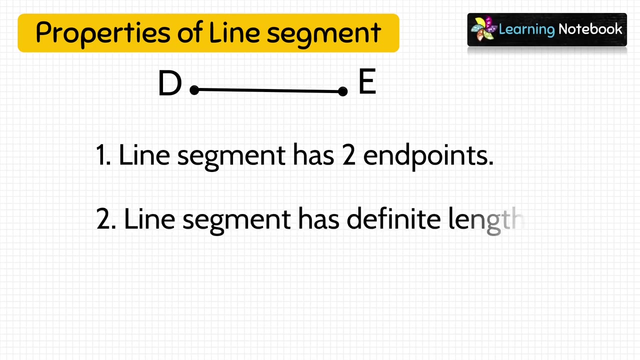 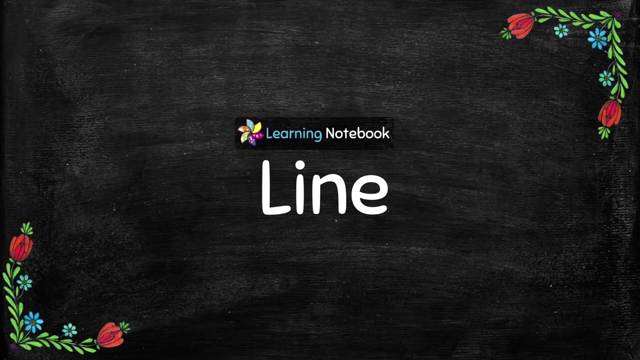 So, students, we have learnt two properties of line segment. First is line segment has two endpoints, Like here, D and E are two endpoints of line segment, DE. And the second property is that the line segment has definite length. Now let's learn about what is line. 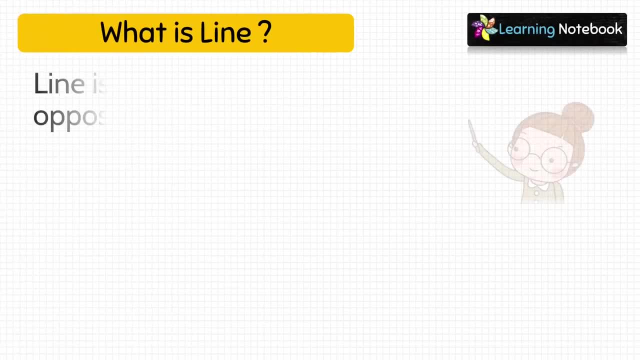 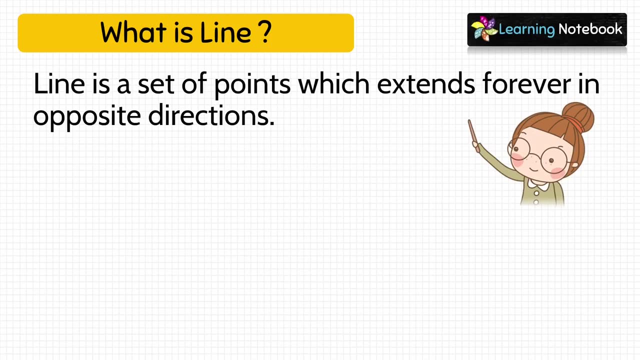 A line is a set of points which extends forever in opposite directions. For example, this is a line. The arrow on its both sides represent that a line goes indefinitely in opposite directions. So, students, it means a line has no fixed length. 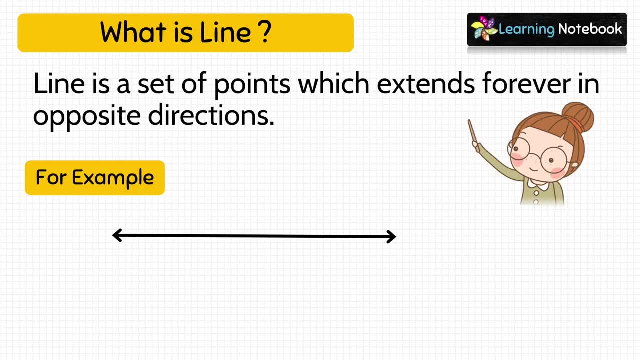 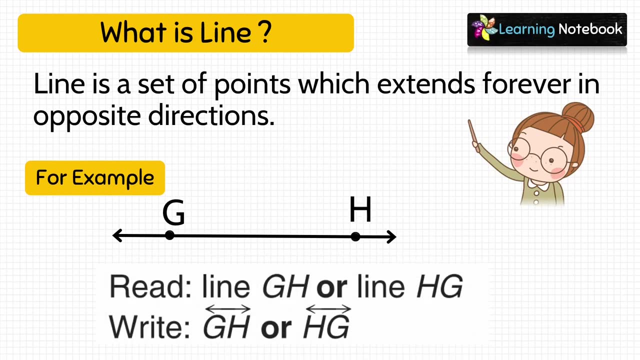 Now let me tell you how to read and write a line. For this we need to take two points. Let's take G and H, So we read a line as Line GH or Line HD. Both the ways are fine. Similarly, we can write it as GH or HD, with a small line drawn on it. 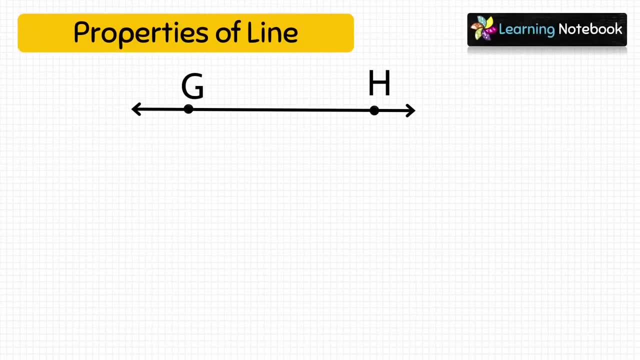 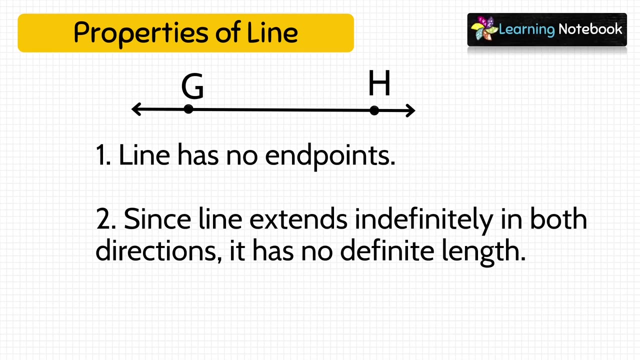 So what properties have we learnt about line Let's revise? First is: a line has no endpoints, Like here in line GH, there are no endpoints. And second property is: since line extends indefinitely in both the directions, so line has no definite length. 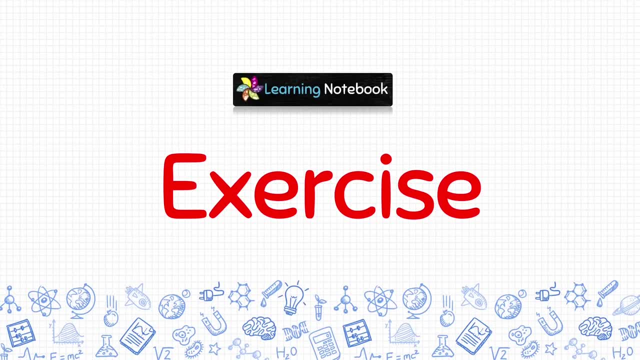 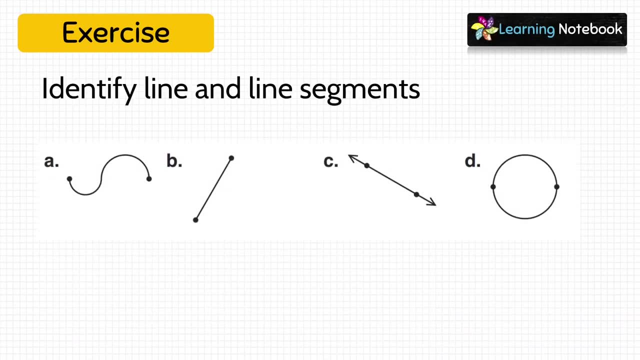 Now let's do some exercise Here. we need to identify line and line segments First. take a look at figure A. A is not a straight path, So it is neither a line segment nor a line. Now take a look at figure B. 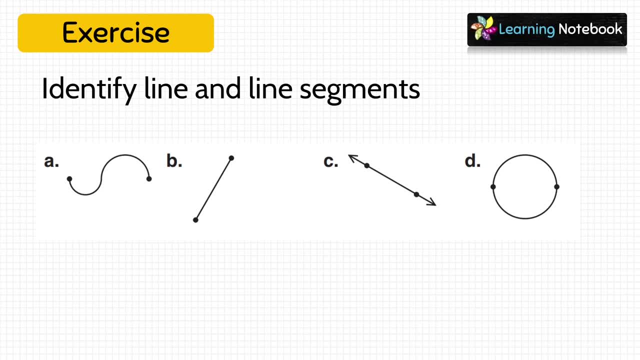 It has two endpoints and has a definite length, So it means it is a line segment. Next, look at the figure C. It has two arrows, So it means it is never ending. Therefore it is a line. And the last figure: 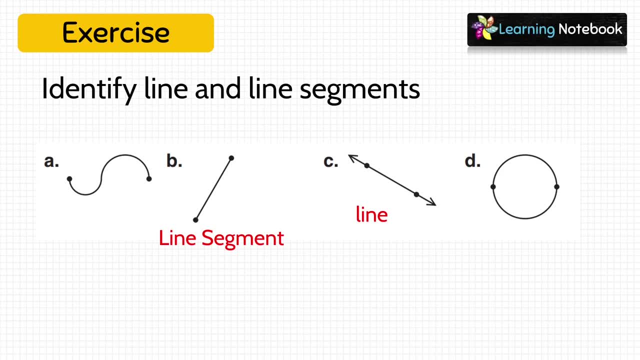 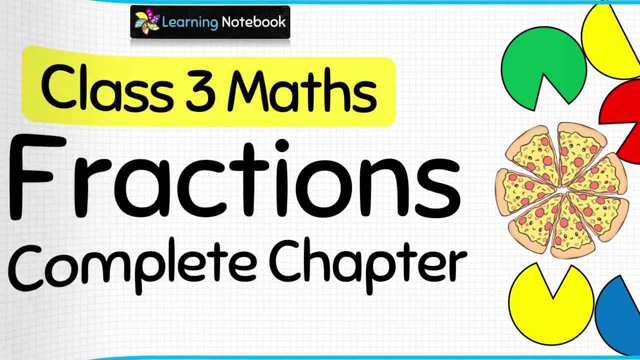 Again, the last figure is not a straight path, So it is neither a line segment nor a line. So, students, now I hope you have understood the difference between line and line segments. We also have separate videos on complete chapter of fractions for class 3.. 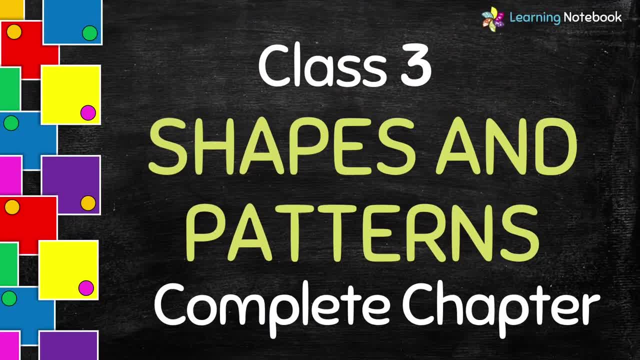 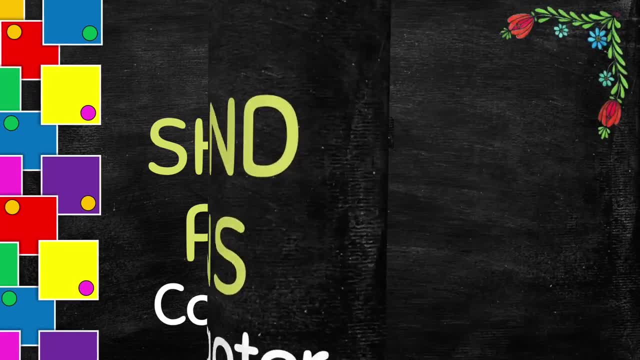 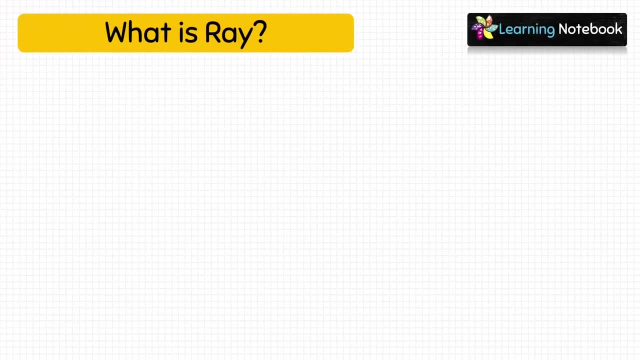 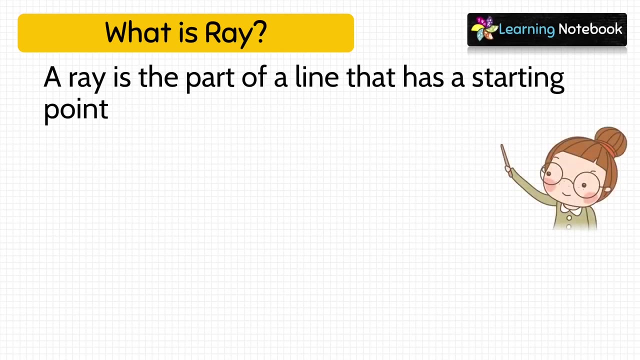 And then you can also learn about shapes and patterns for class 3.. The links to both these videos are below in the description box. Now our next topic is way. A way is a part of the line that has a starting point, and it goes on forever in one direction. 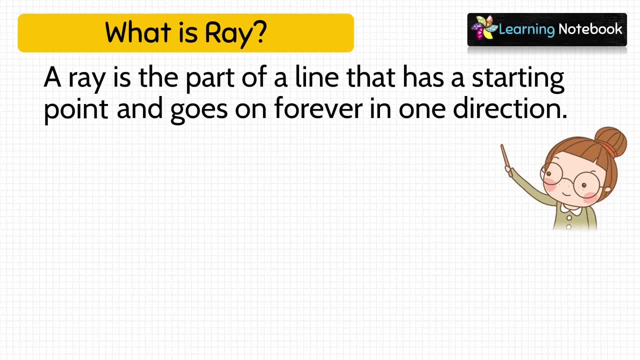 It means way also has no fixed length. It cannot be measured. For example, this is a ray. It has a starting point called K And it goes indefinitely in one direction, towards J. Now let me show you how to read and write way. 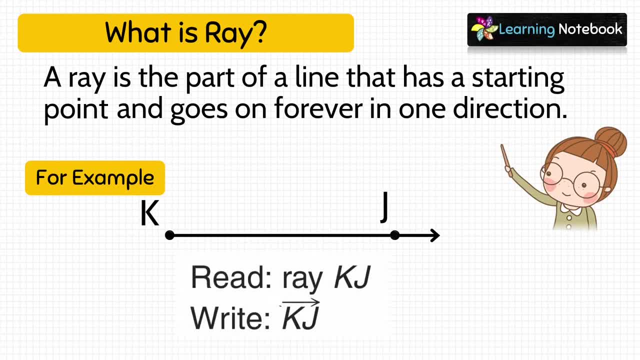 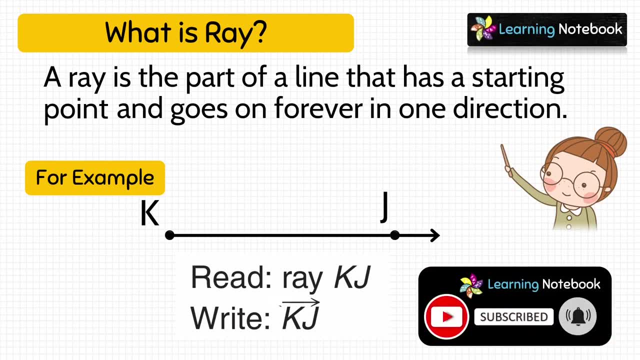 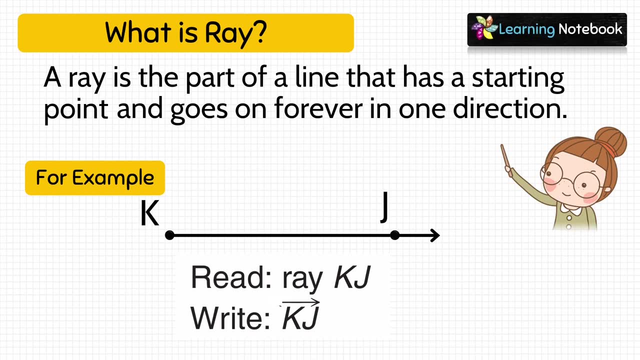 We will read the starting point first, So it will be read as way, KJ. Thus, students, there is only one way to read way, That is, by reading the starting point first. And now how to write it. We will write it, KJ, with a small way drawn over it. 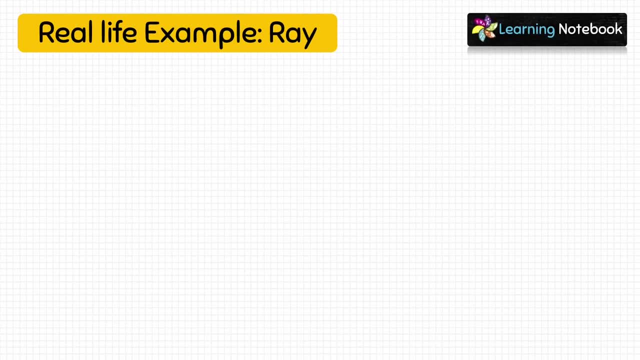 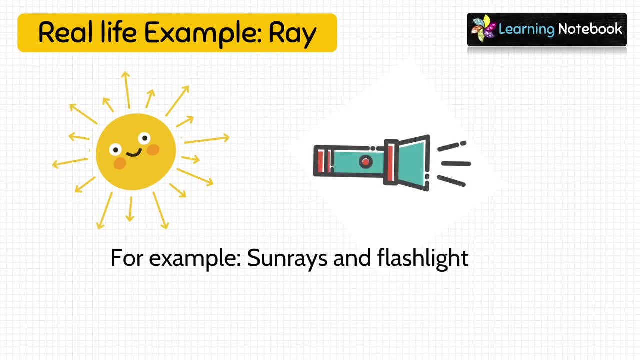 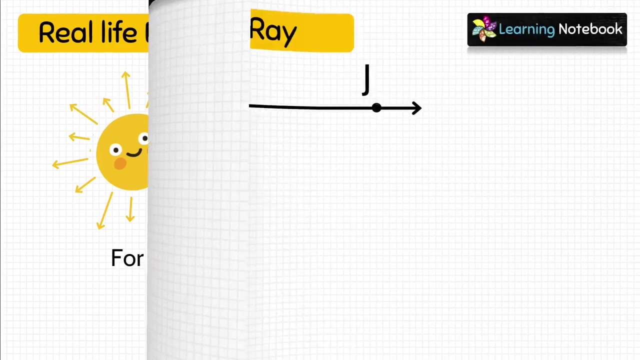 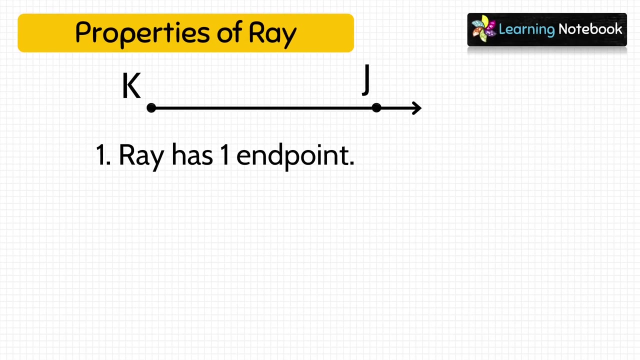 Now let's see some real life examples of way: Ways from sun and ways from flashlight. These are examples of way Because they have a starting point and they go indefinitely in one direction. So what are properties of way? First is a way has one end point. 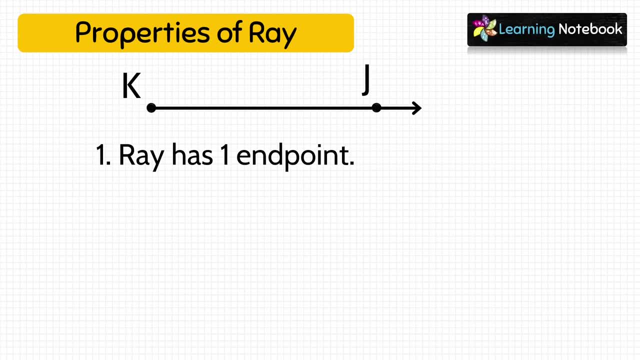 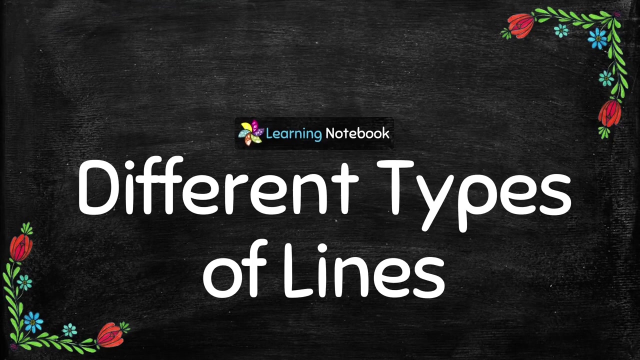 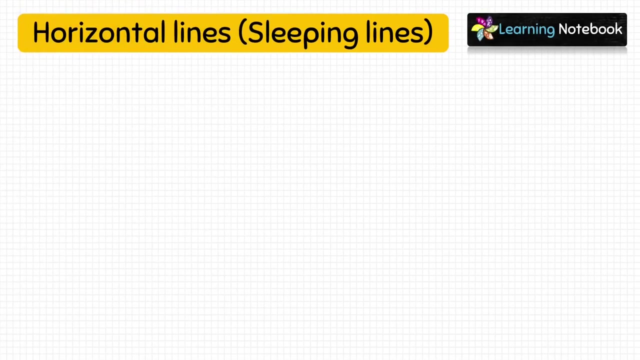 Like here, K is the end point of this way And second property is way has no definite length Because it can extend in one direction indefinitely. Now let's learn different types of lines. So first type of line is horizontal line. 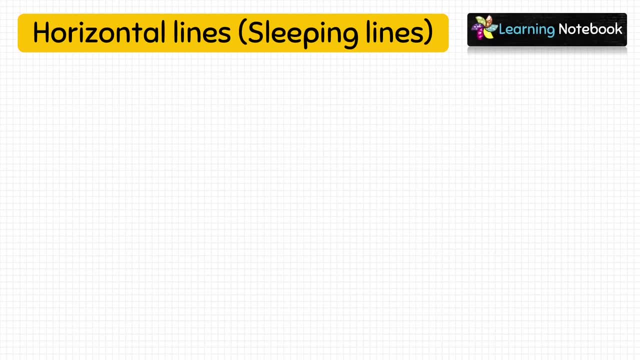 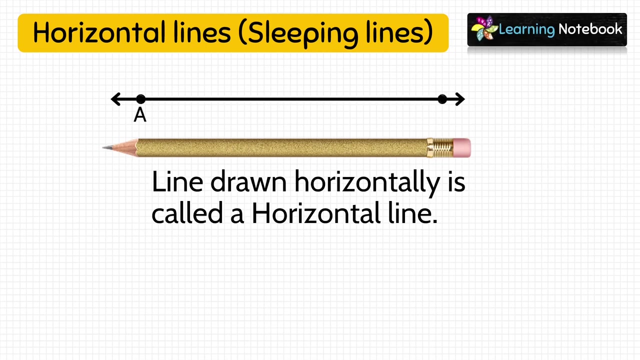 Or we can call it sleeping line, Like here, this pencil is lying flat on the ground. Or we can say that this pencil is lying horizontally. Similarly, a line drawn horizontally is called a horizontal line. Like here, this line AB is drawn horizontally. 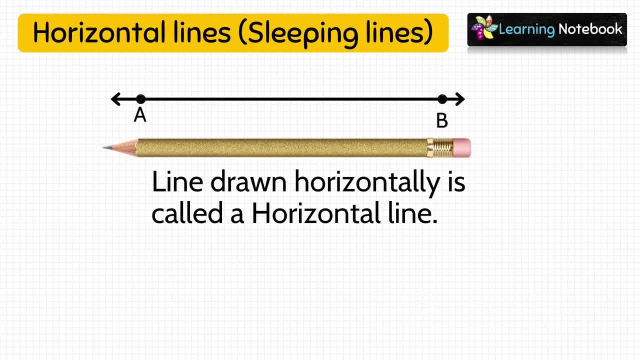 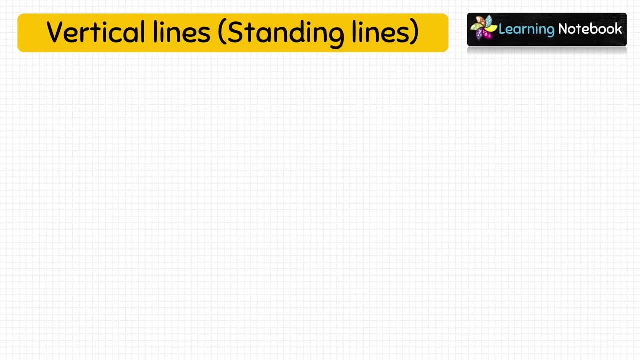 And therefore it is a horizontal line. Now let's understand second type of line, which is vertical line, Or we call it as standing line. Look at this flag mast. It is standing on the ground, Or we can say it is standing vertically on the ground. 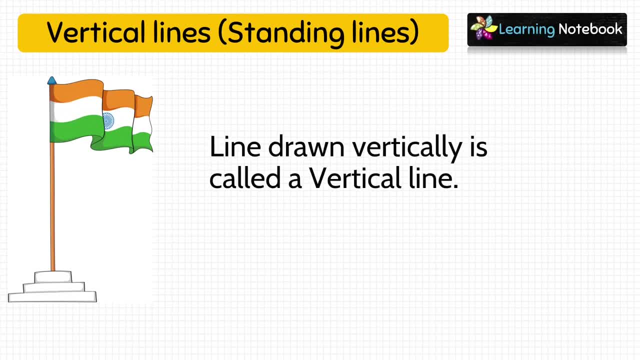 Similarly, a line which is drawn vertically is called a vertical line. Like here, CD is drawn vertically, So it is a vertical line. So students do remember: anything which is lying flat is said to be in a horizontal position, While anything standing straight upright is said to be in a vertical position. 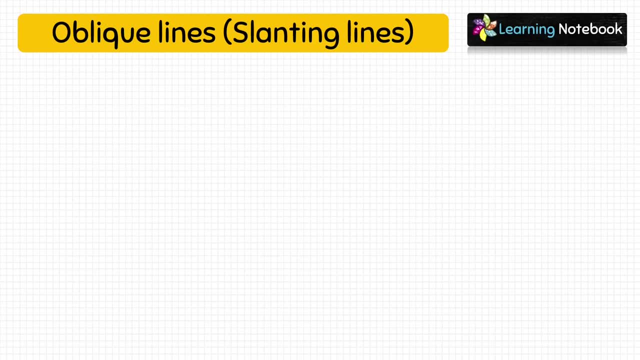 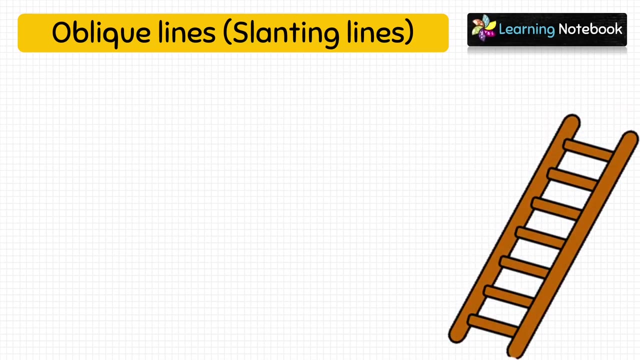 Now the third type of line is oblique or slanting line. A line which is neither horizontal nor vertical is called an oblique or a slanting line. Let's take an example. Look at this figure of a ladder on a vertical wall. 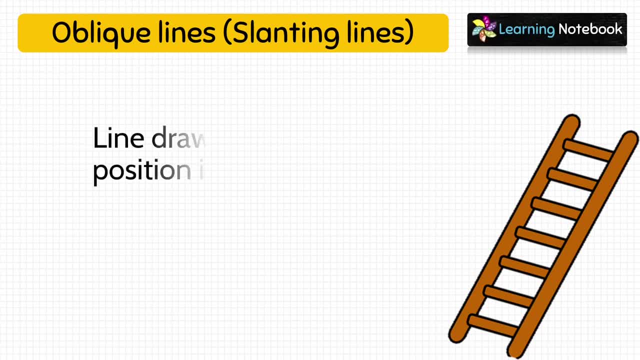 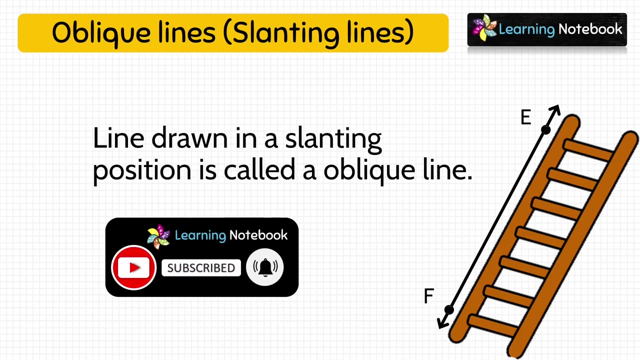 It is in a slanting position, So a line which is drawn in a slanting position is called an oblique line. Here line EF is drawn in a slanting position, So EF is an oblique line. 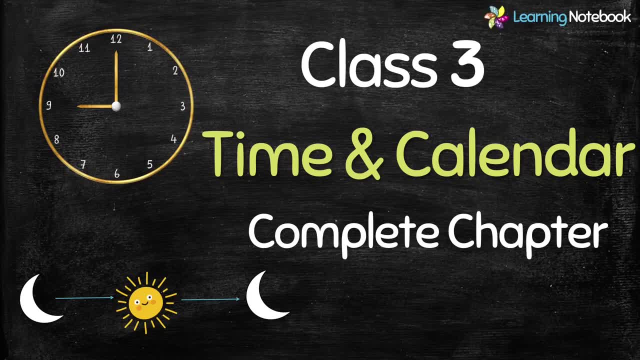 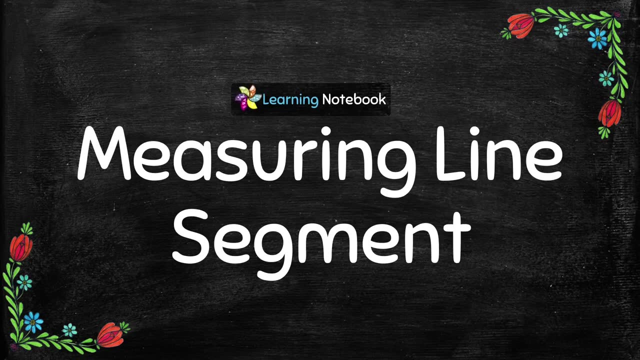 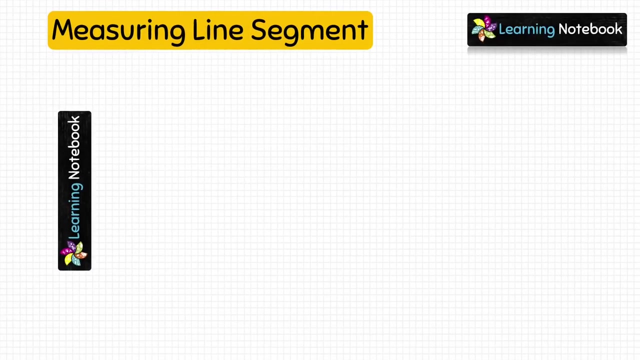 Students. to understand time and calendar for class 3, you can refer to our separate video. The link to this video is below in the description box. Now let's move to our next topic: measuring line segment Students. we measure the length of a line segment. 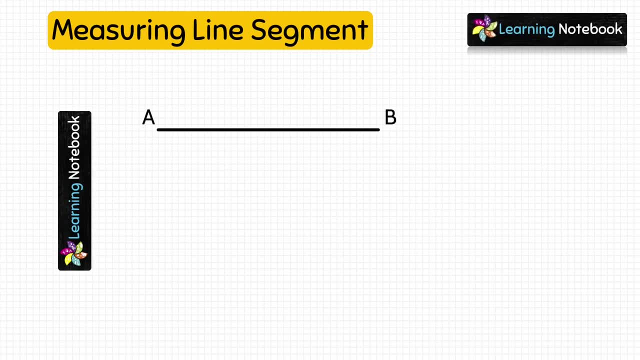 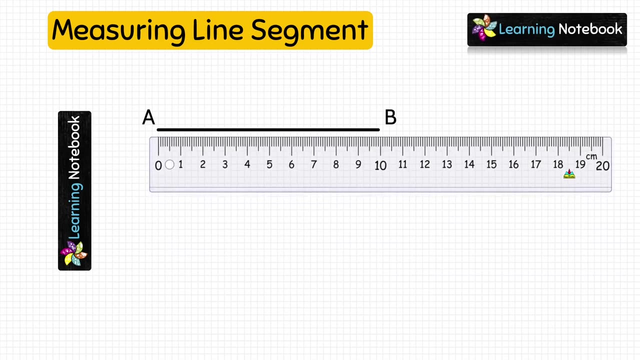 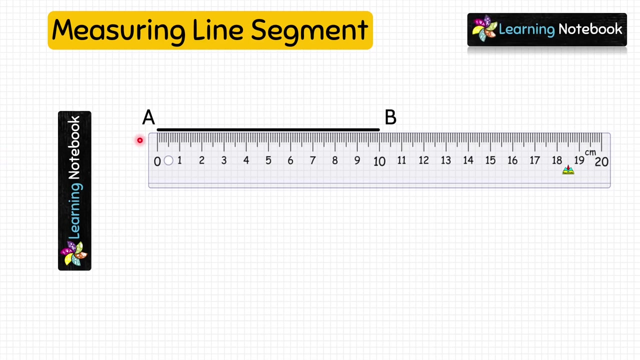 with the help of a ruler Here, let's measure the length of this given line segment AB. For this let's take a scale and place it along the line AB, such that 0 is at point A. Now see where is point B. 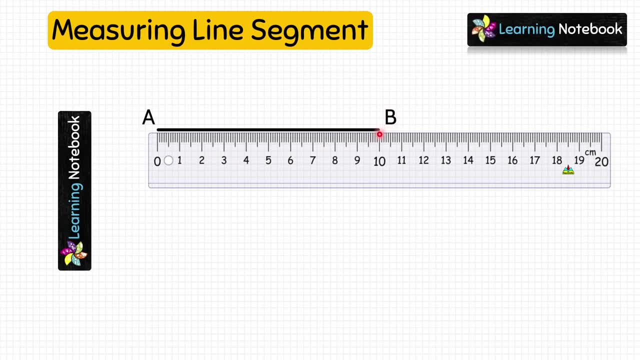 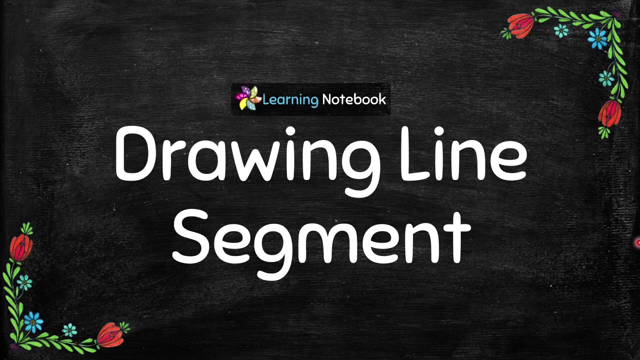 The reading of the scale of point B is 10.. It means length of the line segment AB is 10 cm. So this is how we measure length of a line segment. Now let's learn how to draw a line segment. Now to draw a line segment. 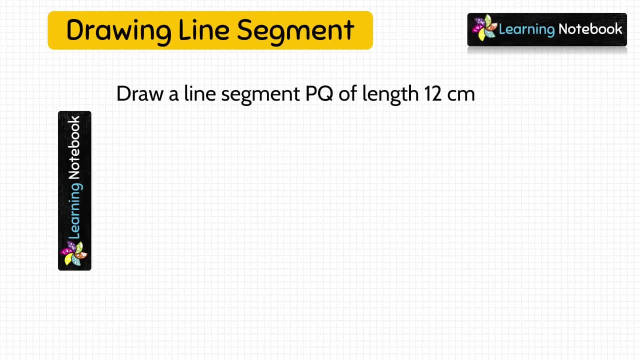 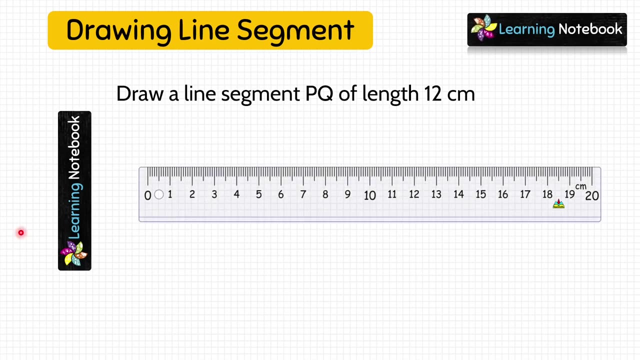 again we will take help of a ruler. Question is: draw a line segment PQ of length 12 cm. So let's take a scale and first mark point P, which is at 0 mark of the scale. So remember first point of a line segment. 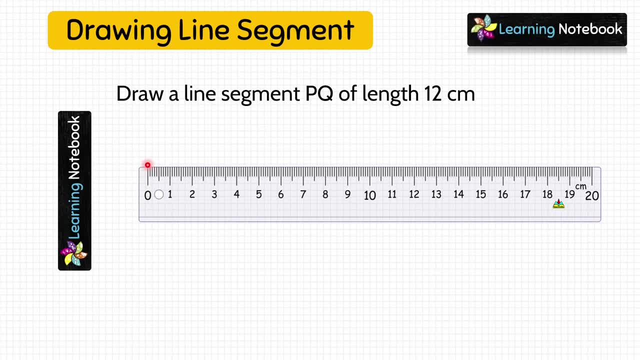 is always 0.. Now, students, we have to draw a line segment of 12 cm. This means we have to mark second point Q at 12 cm, mark of the scale. It is here, As you can see, the pointer 12 cm is here. 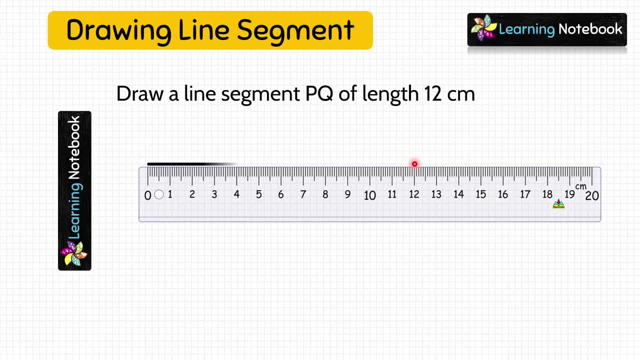 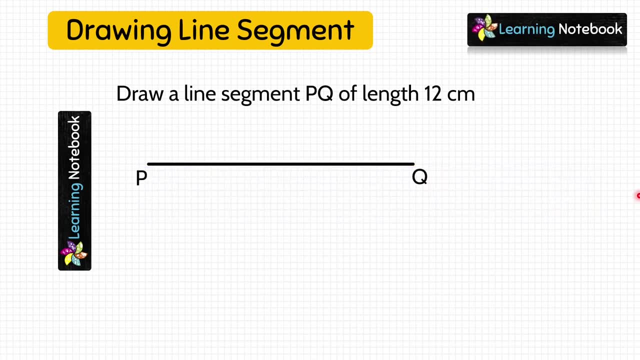 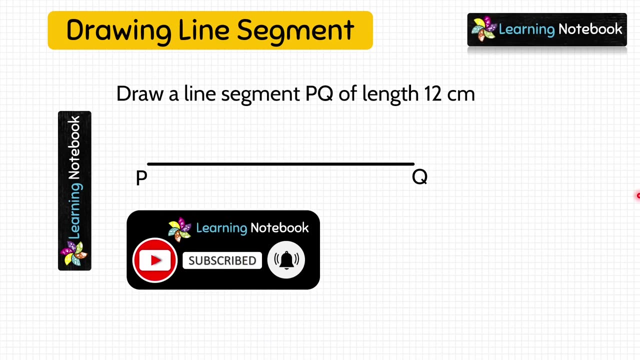 And lastly, we will draw the line segment joining both these points to form line segment PQ of length 12 cm. So this is how we can draw a line segment of any length. Question is how to draw a line segment PQ of length 12 cm. 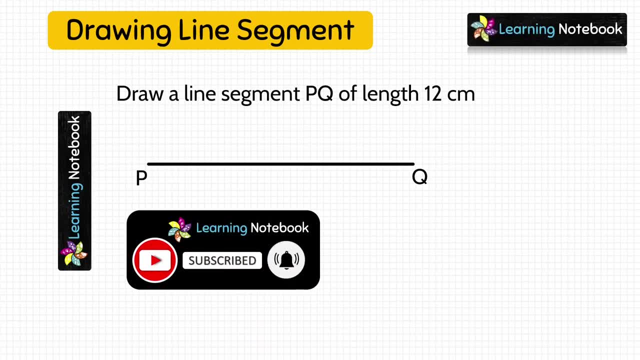 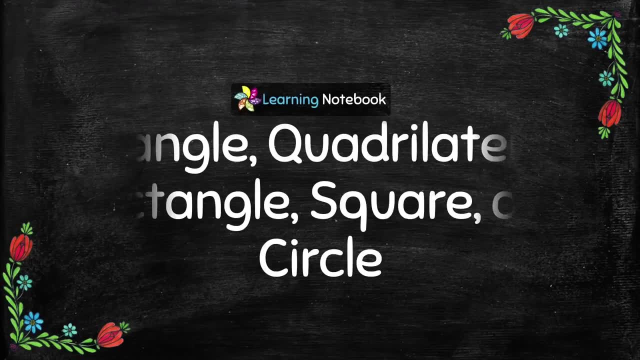 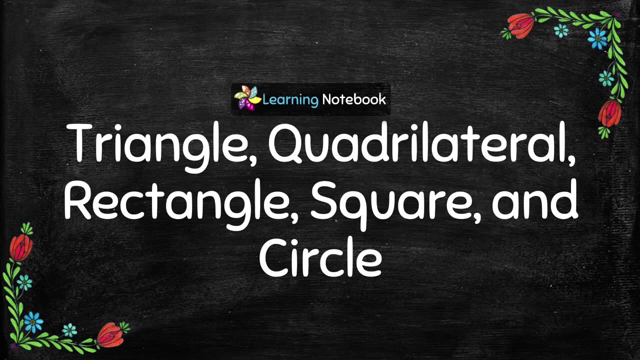 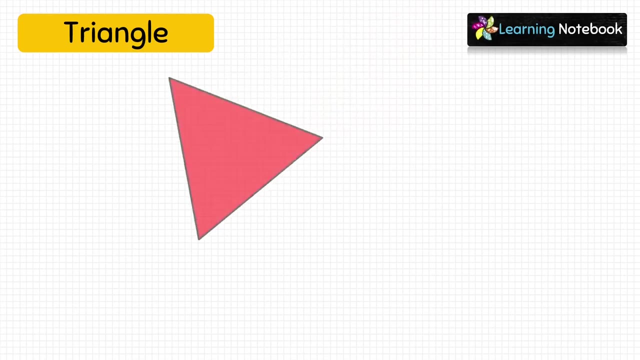 If you still not have subscribed to our channel Learning Notebook, then do subscribe it And make sure to press the bell icon. Now let's move to our next topic: Triangle, quadrilateral, rectangle, square and circle. First let's understand. 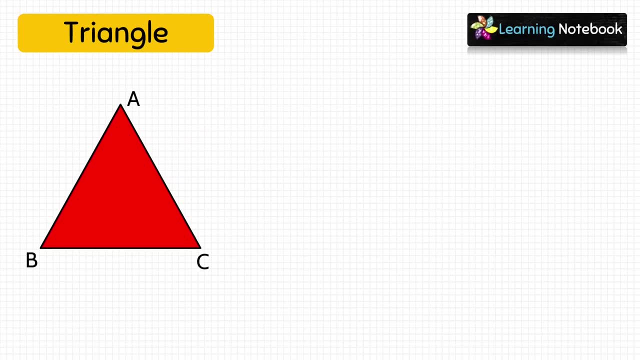 what is a triangle? A figure formed by three line segments is called a triangle. Look at this figure. It is formed by three line segments, So it is a triangle. We will call it as triangle AB. Next, It is a triangle. 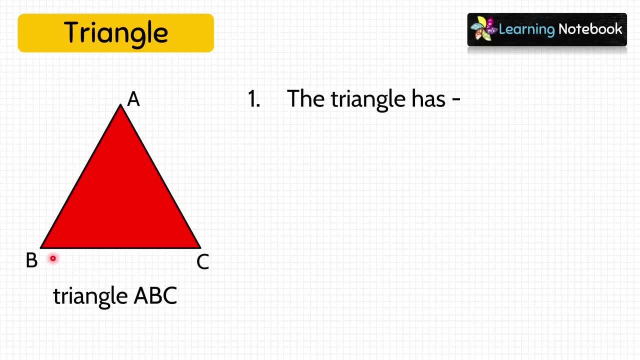 with three lines, Because triangle has three lines. For example, a triangle has Three sides. Now, triangle has three sides. What about triangle C? Next, our triangle has, triangle has three sides. Like here, we have three sides AB. 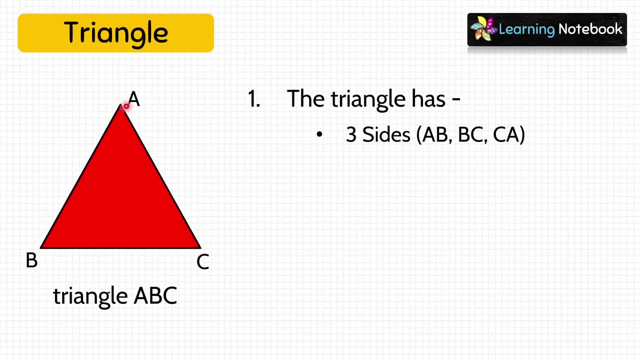 BC and CA. Then our triangle has three sides. Next triangle has Three vertices, or we can call it three corners, Like here. three vertices are A, B and C. Another important point to note is that sides of a triangle may or may not be of equal length. 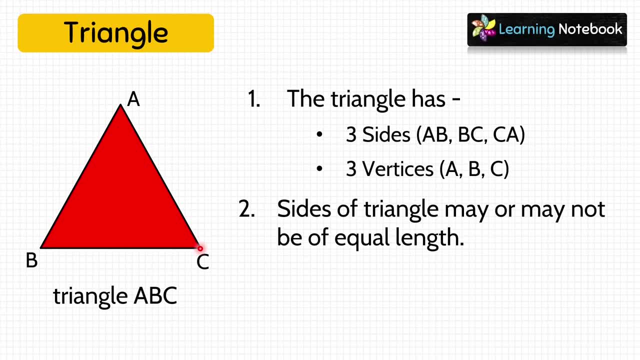 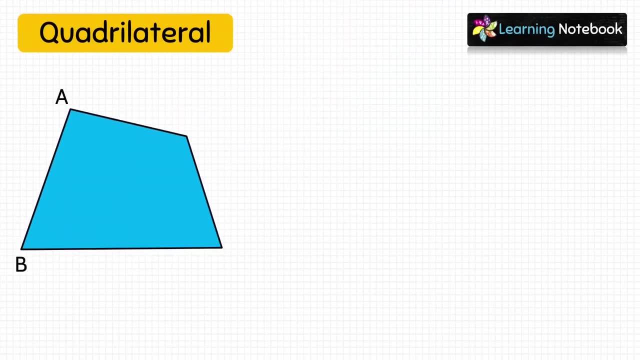 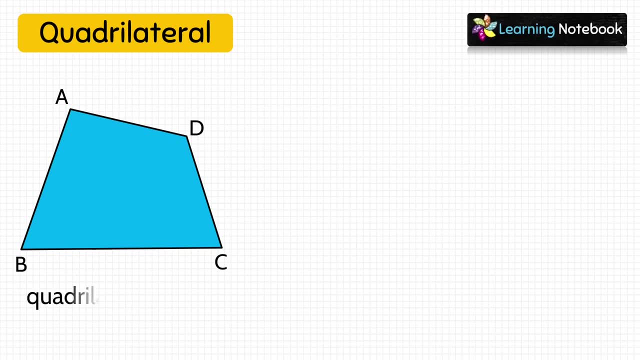 Like here: A, B, C, D is a quadrilateral because it is formed by four line segments. Next, a quadrilateral has how many sides? Yes, four sides. Look here: A, B, B, C, C, D and D A. 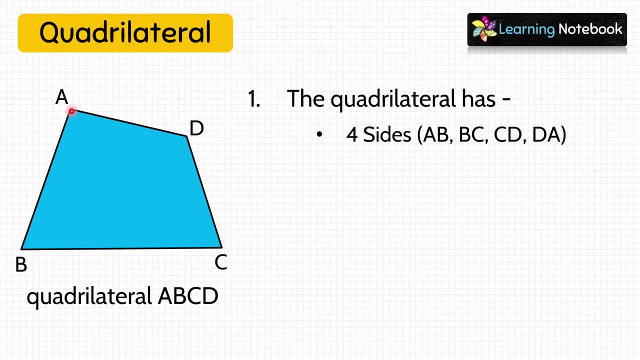 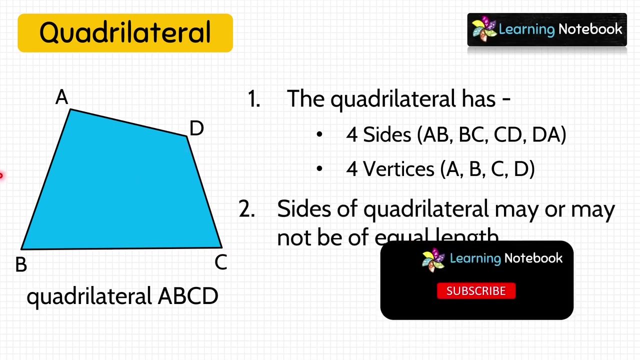 These are four sides of this quadrilateral- A, B, C, D- And then it has four vertices or four corners: A, B, C, D, B, C and D And, as we learnt in triangle, sides of a quadrilateral may or may not be of equal length. 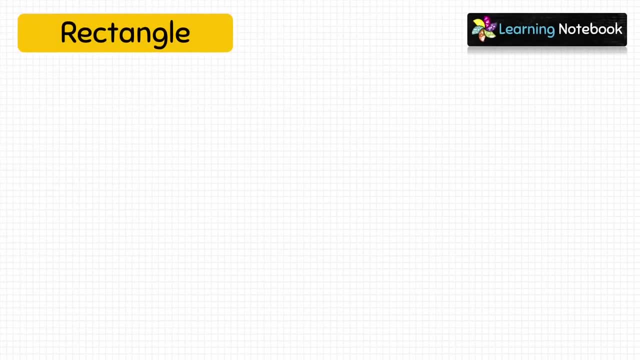 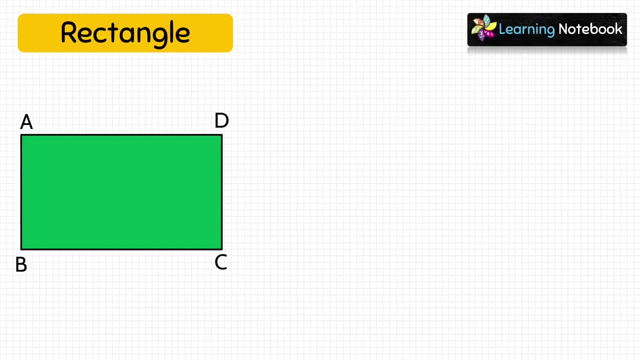 Now, next shape is rectangle, Which is a quadrilateral By, Because rectangle is formed by four line segments And a rectangle has how many sides? Four sides. So here in this rectangle- A, B, C, D- four sides are: A, B, B, C, C, D and D. 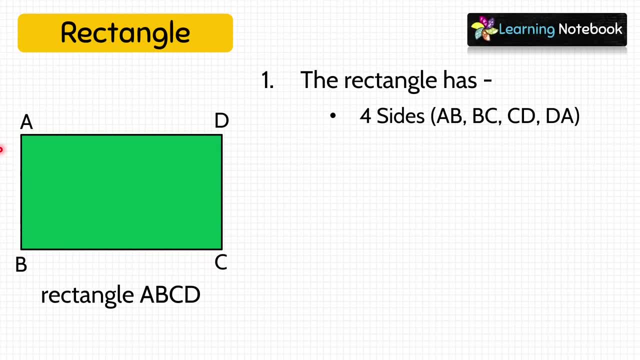 So here in this rectangle A, B, C, D. So here in this rectangle A, B, C, D and D. So here in this rectangle A, B, C, D and D. So here in this rectangle A, B, C, D and D. 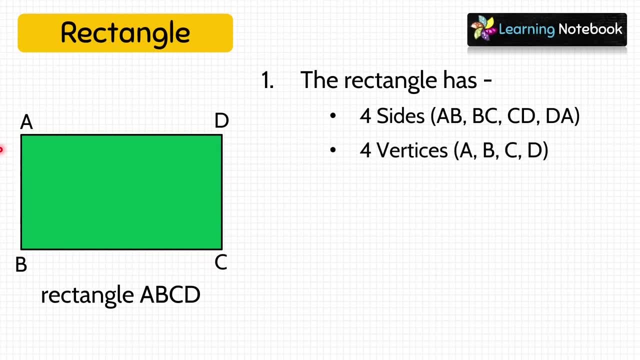 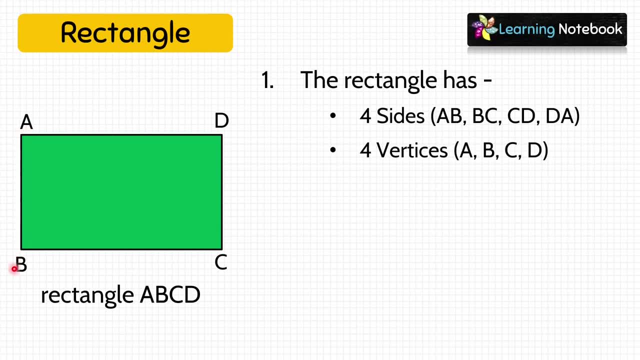 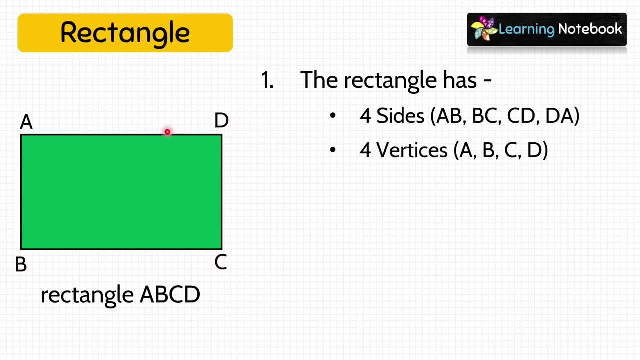 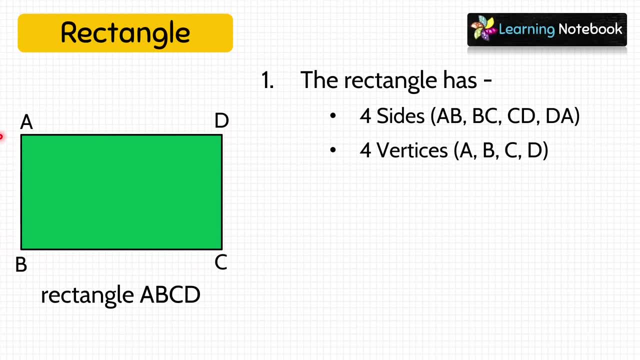 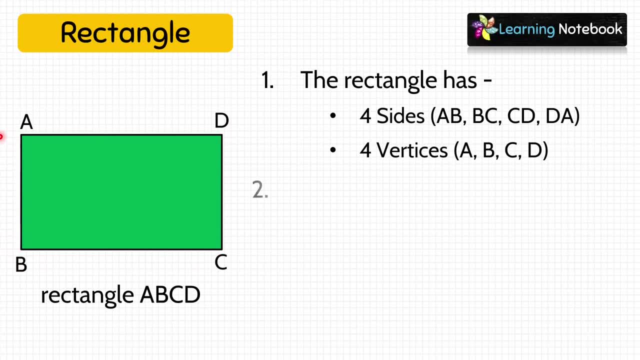 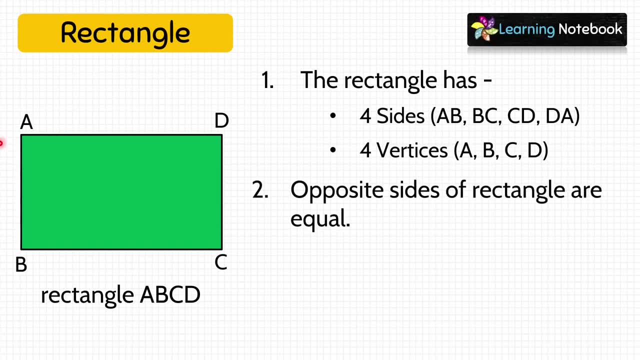 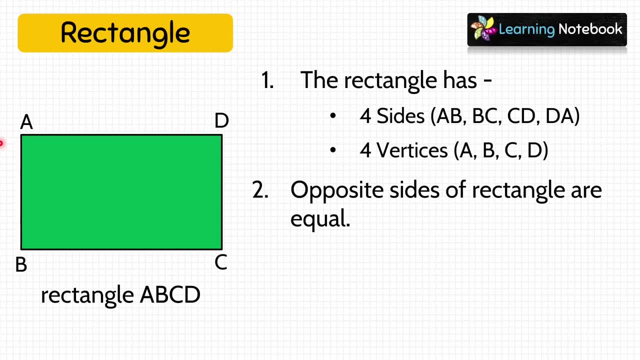 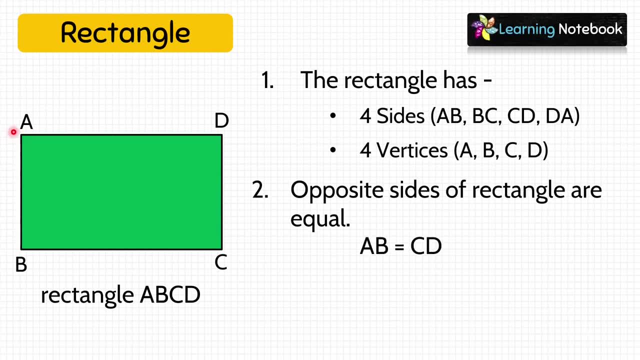 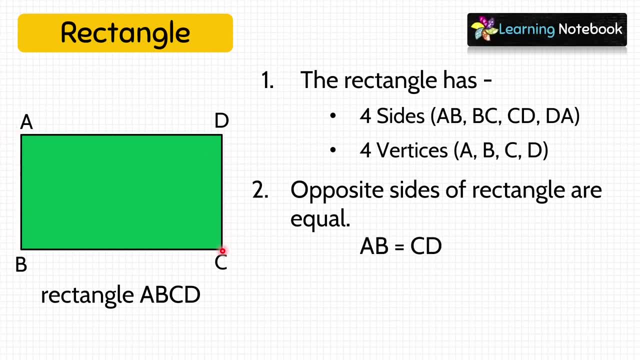 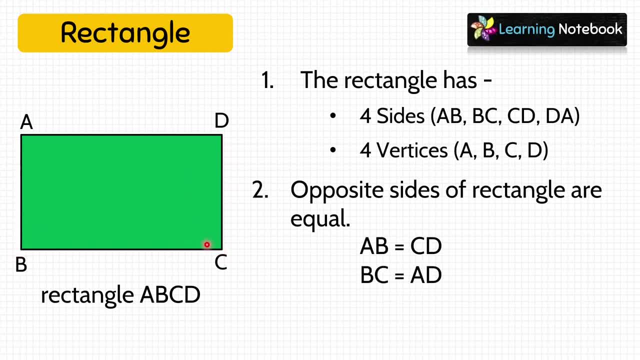 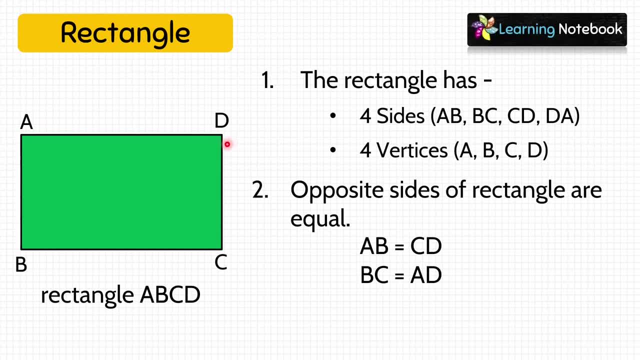 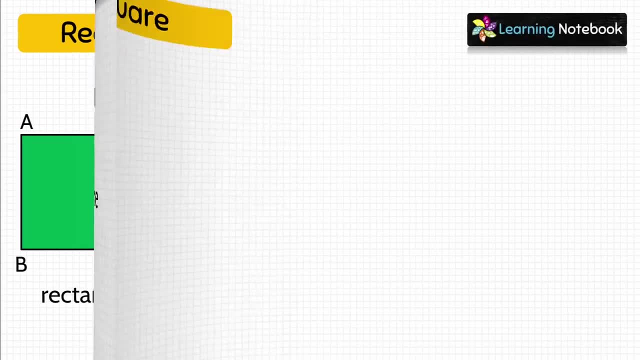 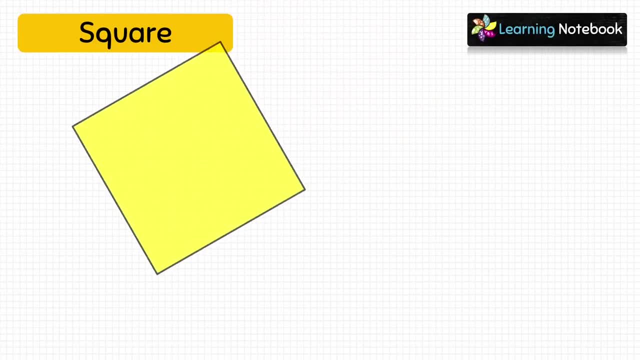 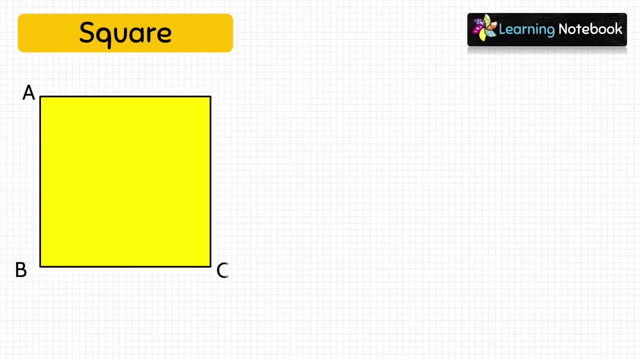 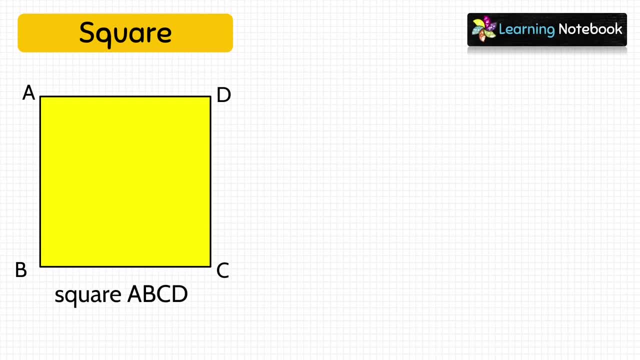 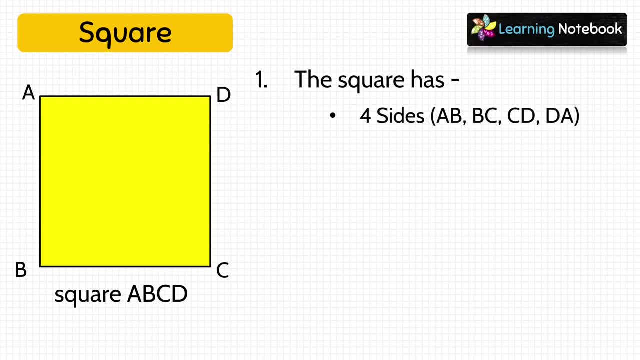 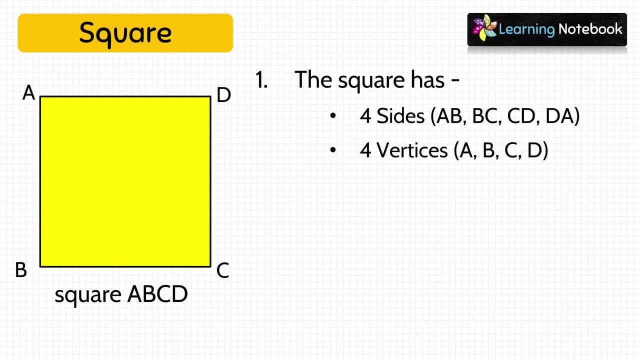 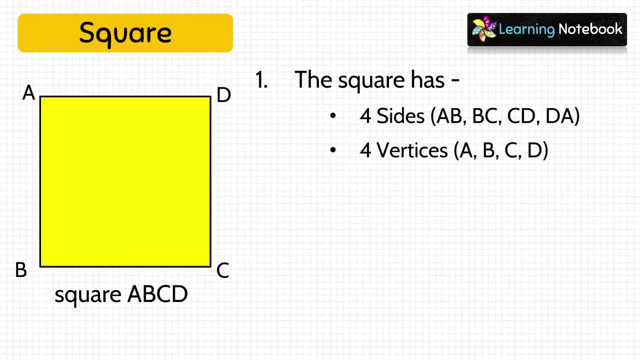 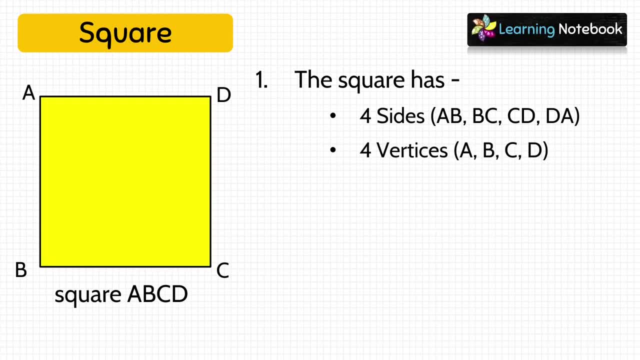 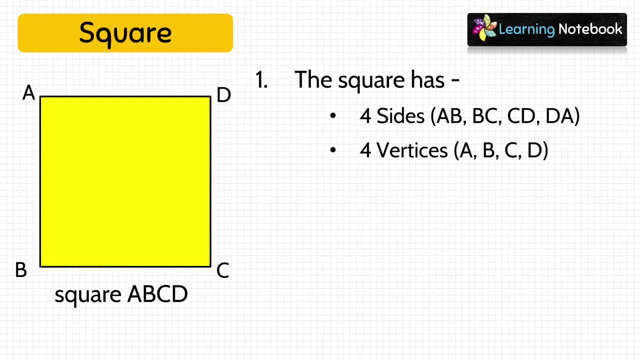 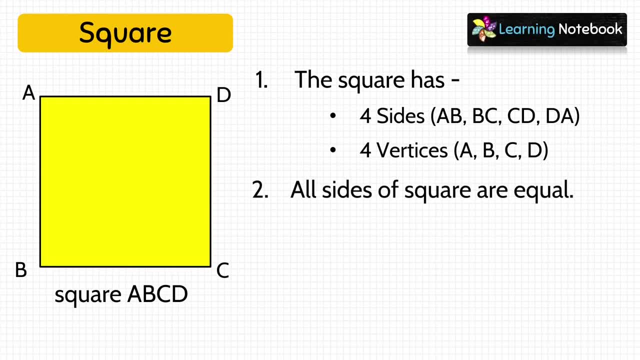 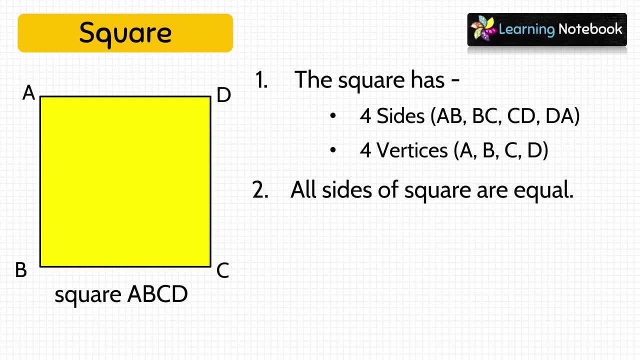 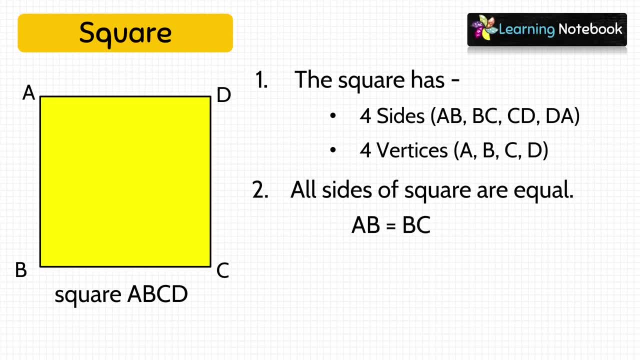 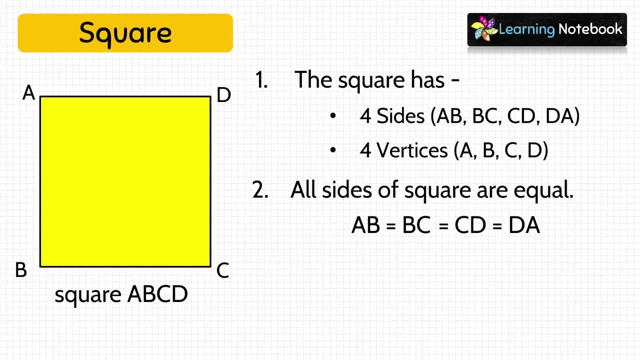 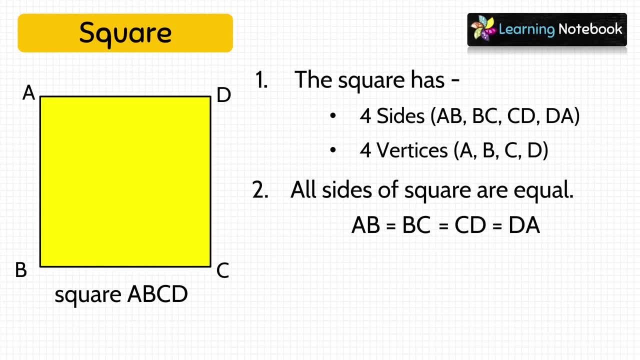 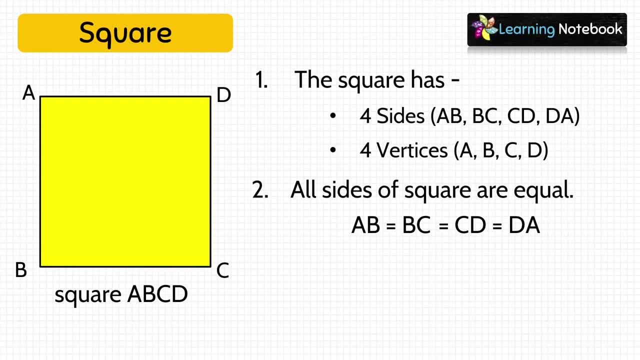 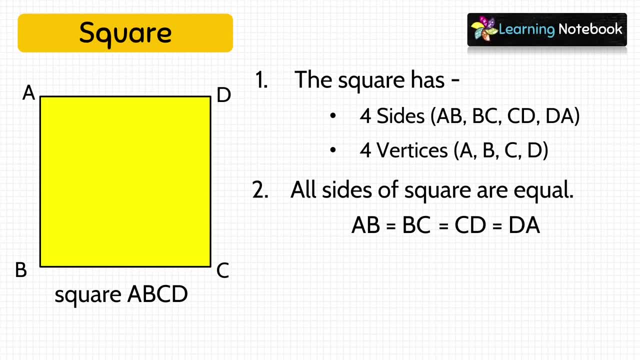 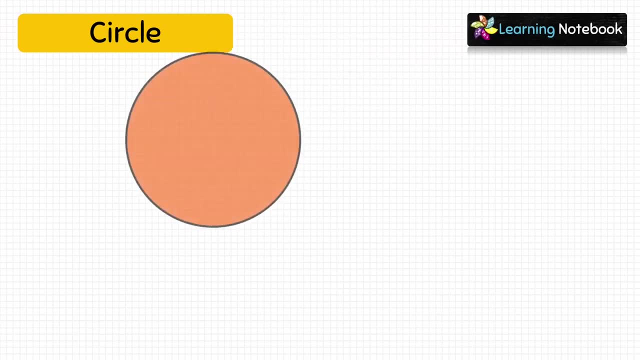 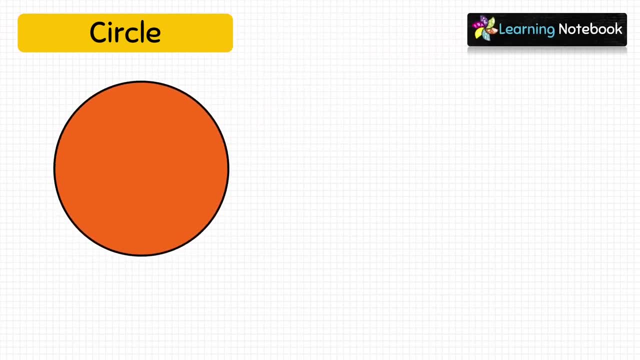 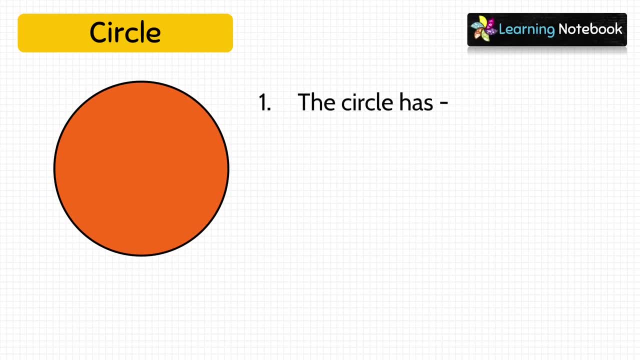 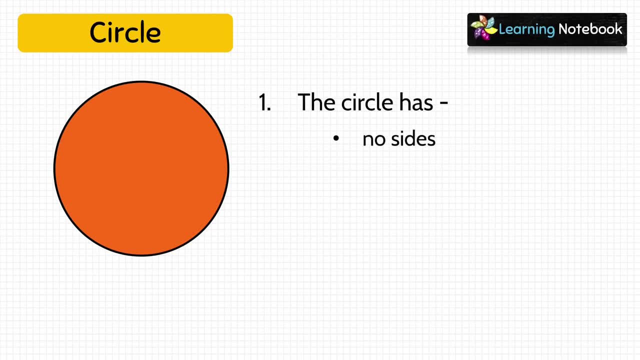 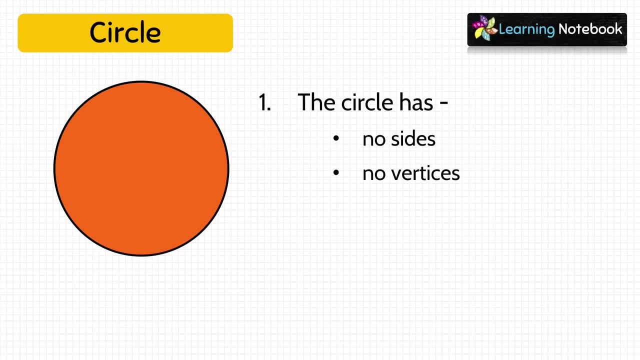 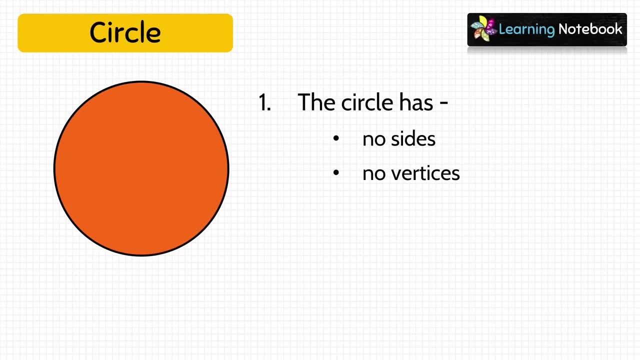 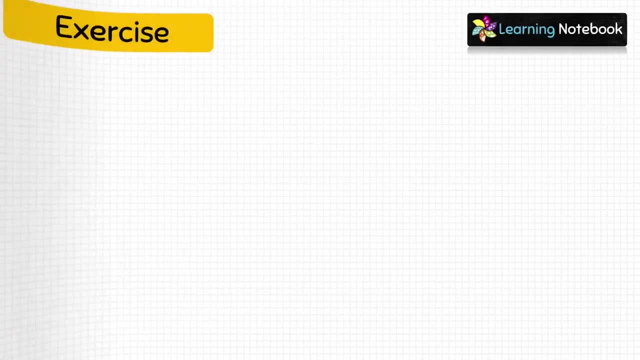 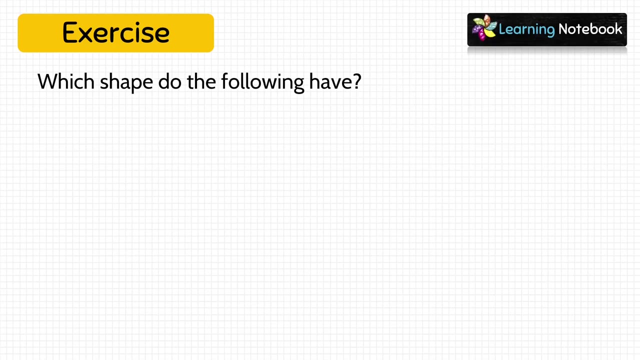 So this was all about plane shapes. Now let's do an exercise. Question is: which shape do the following have The wheel of a bicycle? is of which shape? Yes, circle Next. can you tell me what is the shape of a page of the book? 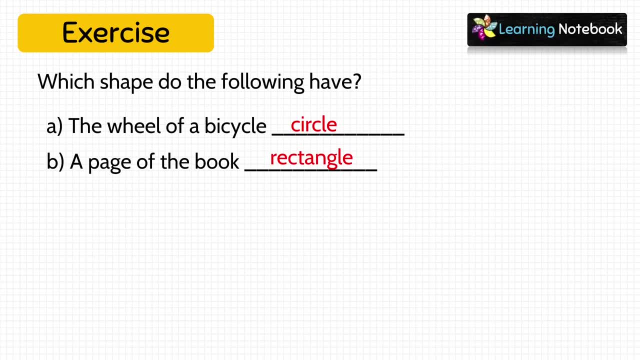 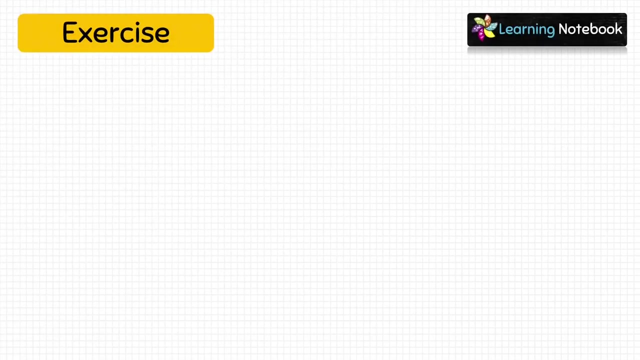 Yes, it is rectangle. Next, a pizza slice. A pizza slice is of triangle shape, And the last is the face of a die. It is of square shape. Let's see the next question. Count the number of triangles in the following figure: 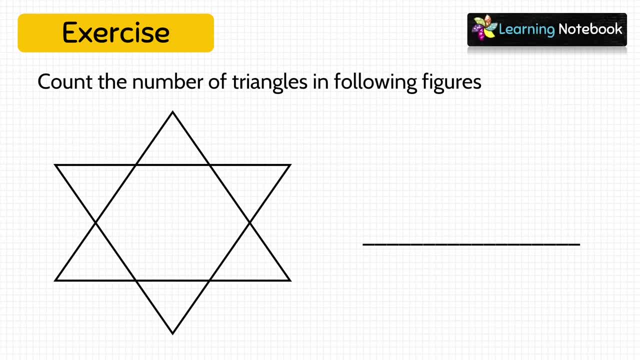 Here we are given with a figure and we have to count the number of triangles. So let's further. First count the small triangles 1, 2, 3,, 4, 5, 6.. So we have 6 small triangles. 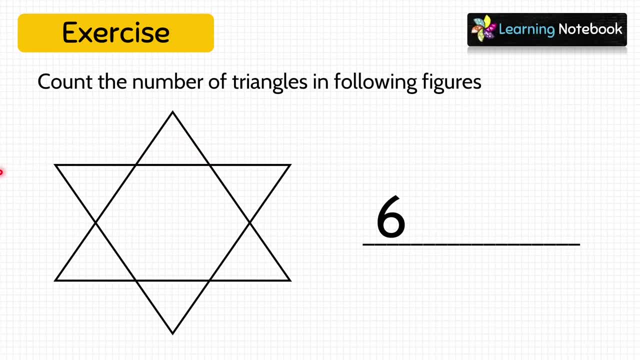 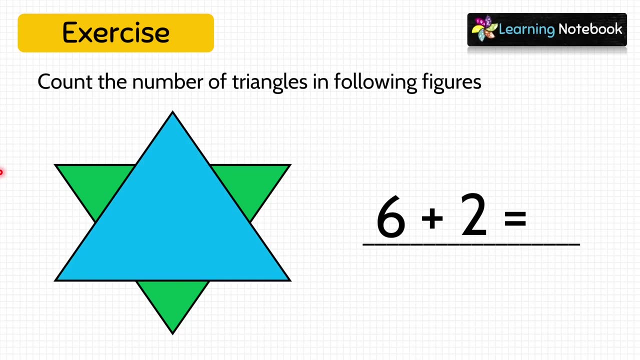 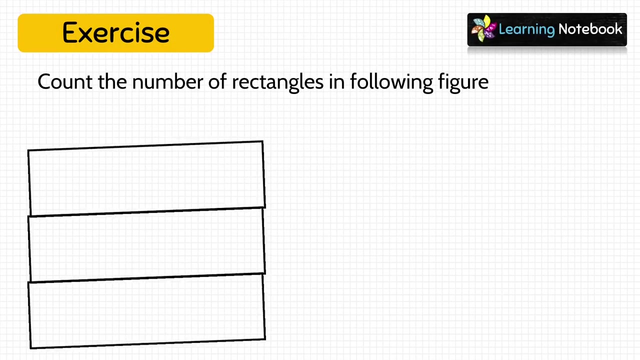 Now look carefully. We also have big triangles. One is this And another one is this. So 6 plus 2 big triangles equal to 8.. So this figure has 8 triangles. Now in the next question we have to count number of rectangles. 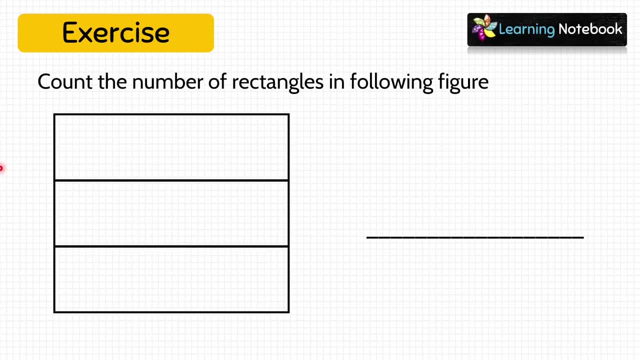 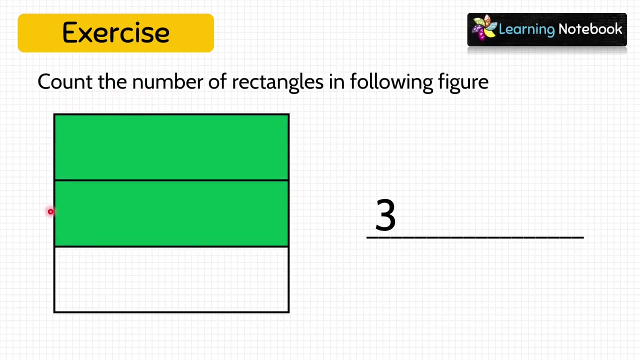 So let's start with counting small rectangles: 1,, 2,, 3.. So let's write 3.. Now let's combine two of these small rectangles to form a big rectangle. So how many such rectangles are there? 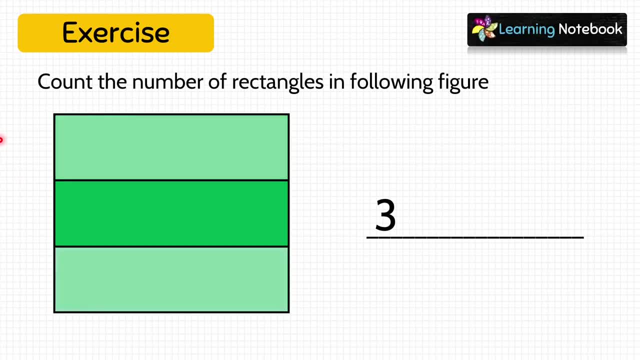 One is this And next one is this. So there are two such rectangles, So let's write 2.. Now we can also form a big rectangle by combining all these three rectangles. This is the big rectangle, Which is only 1.. 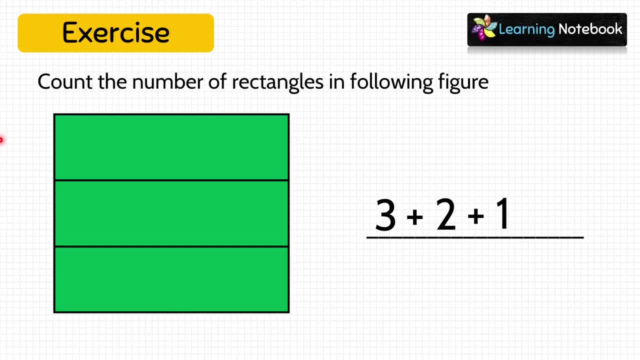 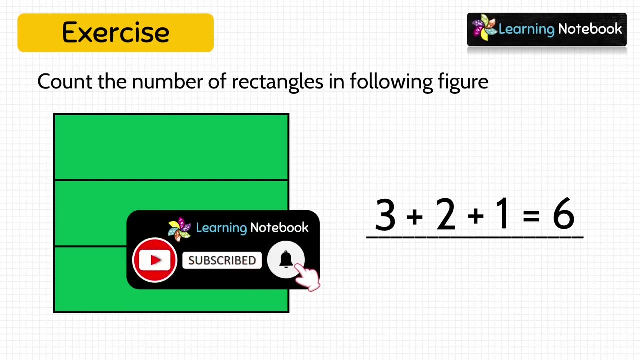 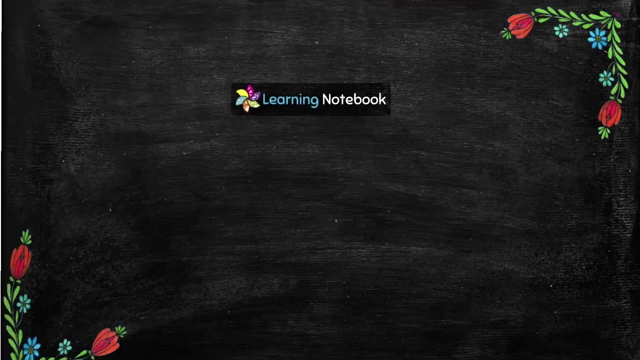 So let's write 1.. So here, total number of rectangles are 6.. If you still not have subscribed to our channel Learning Notebook, then do subscribe it And make sure to press the bell icon. Now let's move to our next question. 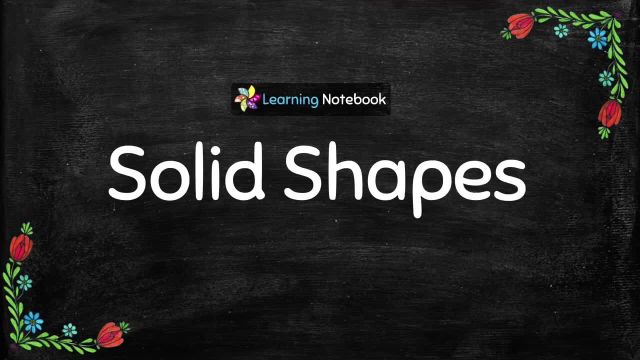 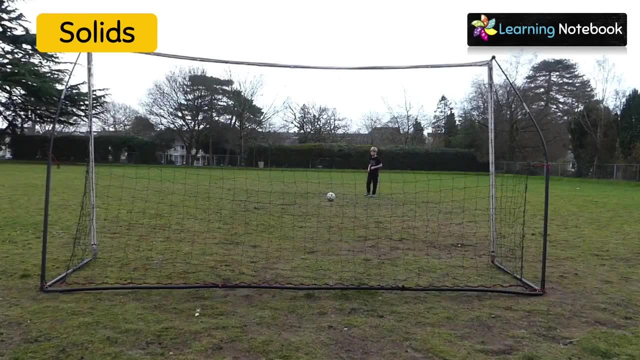 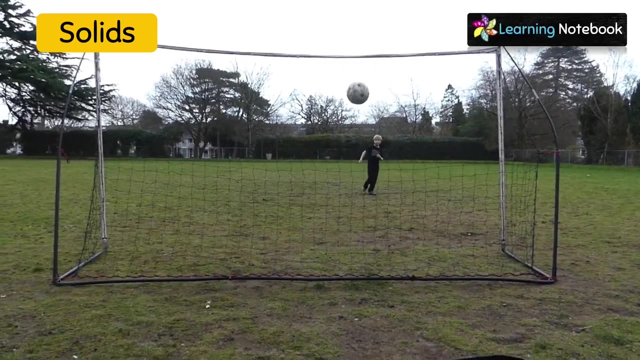 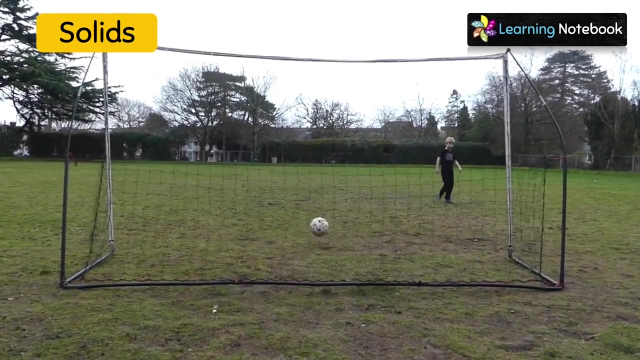 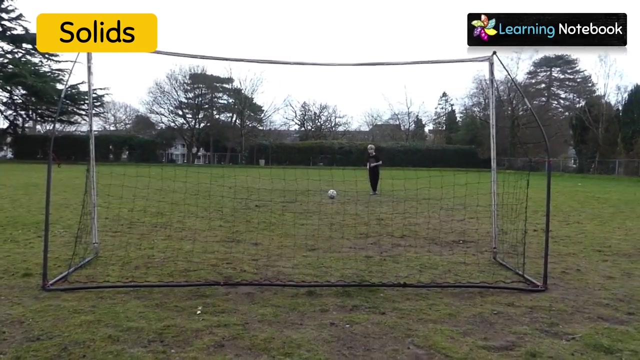 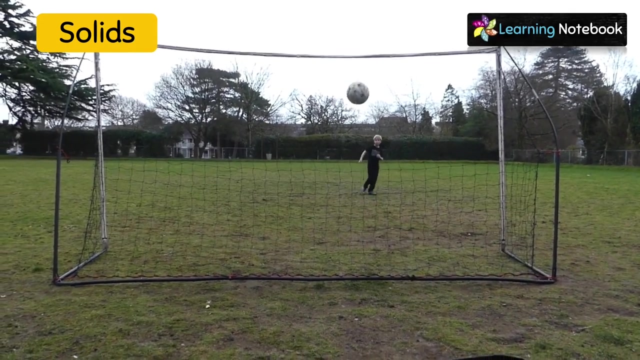 Now let's move to our next topic: solid shapes. First, let's understand what are solids. When we kick a ball, it goes up in the air and it moves in the space. So this ball is called a solid, Because any object that occupies space is called a solid. 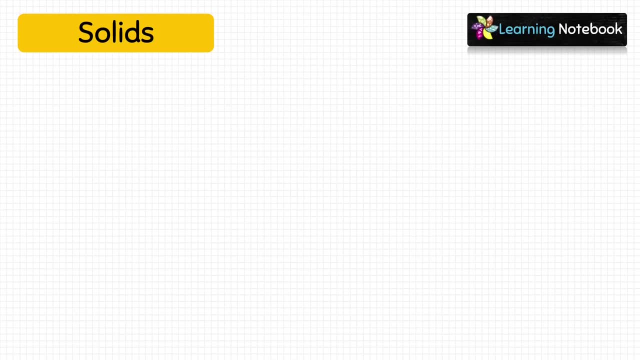 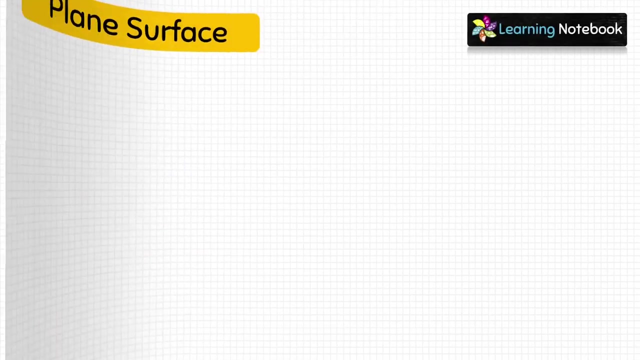 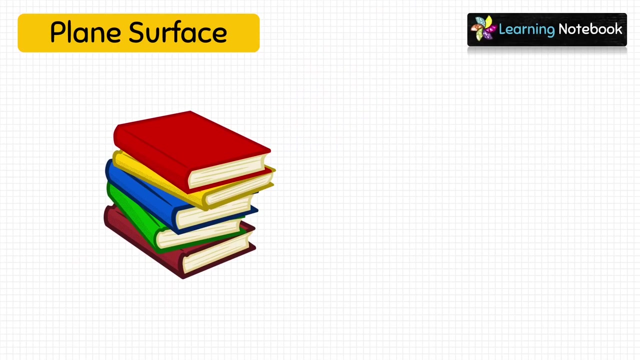 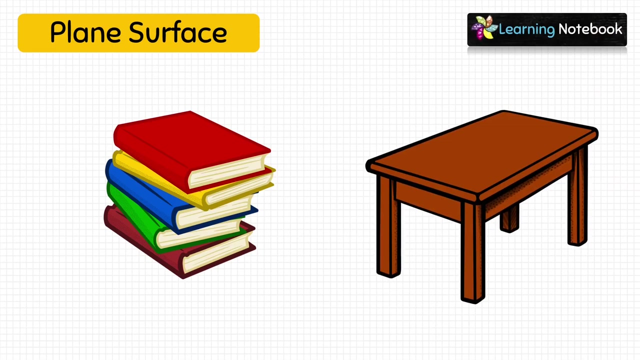 Now, all solids have a surface, And a surface can be a plane surface or a curved surface. Now look at these books. These books have a plane surface Or, we can say, a flat surface. Similarly, look at the top of this desk. 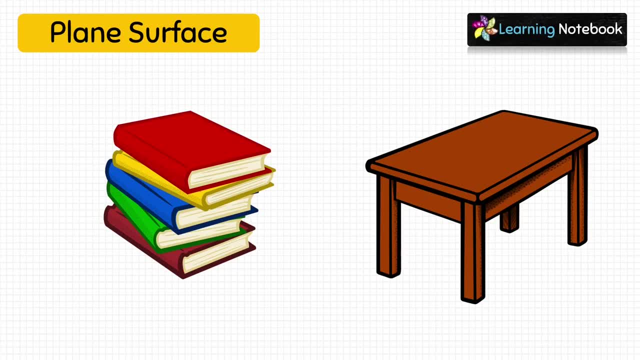 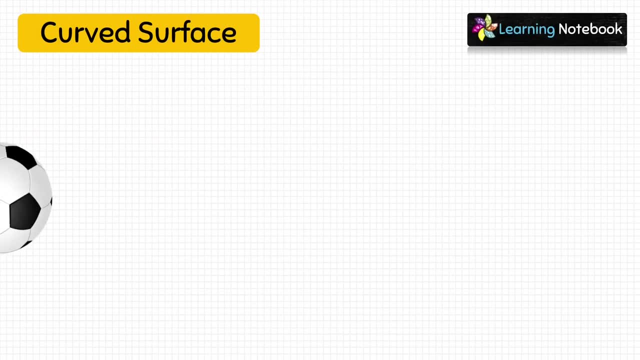 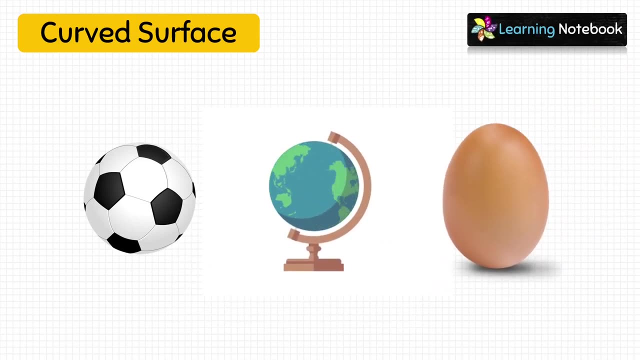 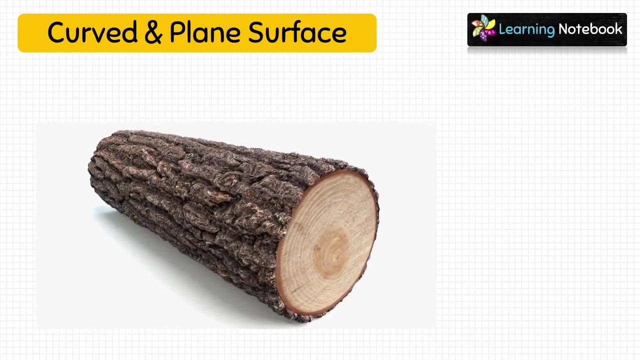 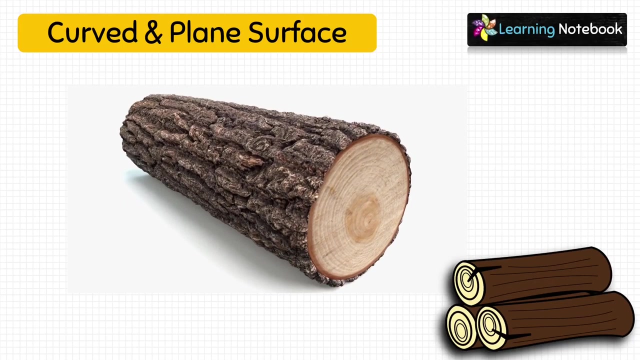 It also has a plane surface. Now students look at this football globe and an egg. All these have curved surfaces, But some shapes have both curved surface as well as a plane surface, For example, if we look at this log of wood. 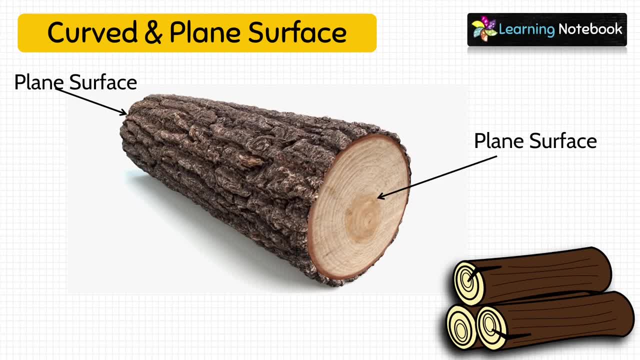 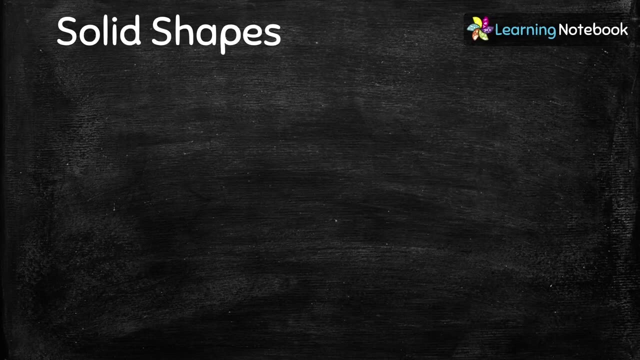 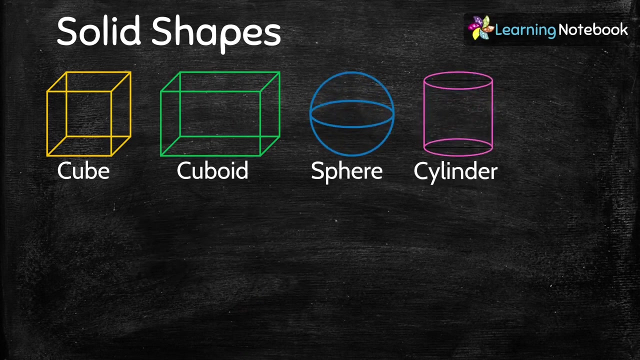 it has two plane surfaces and one curved surface. Now let's learn about solid shapes. These are cube, cuboid, sphere, cylinder and the last solid shape is cone. Now, students, to understand these solid shapes better, let's take few examples of each of them. 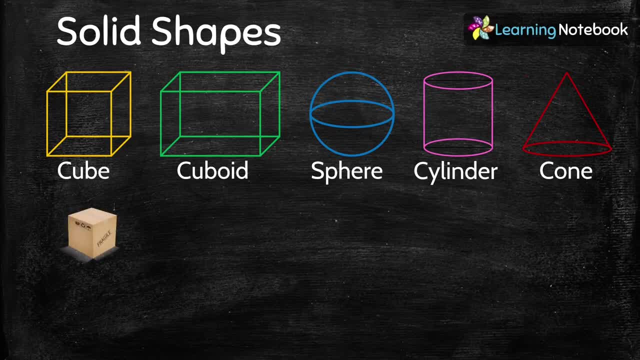 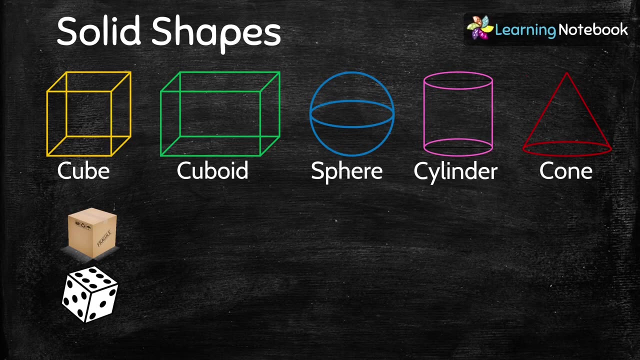 Examples of cube are a carton box and a dice. You must be using dice in your games. This is the best example to remember cube. Now examples of cuboid are a book and a match box. Take your maths book. It is a very good example to remember cuboid shape. 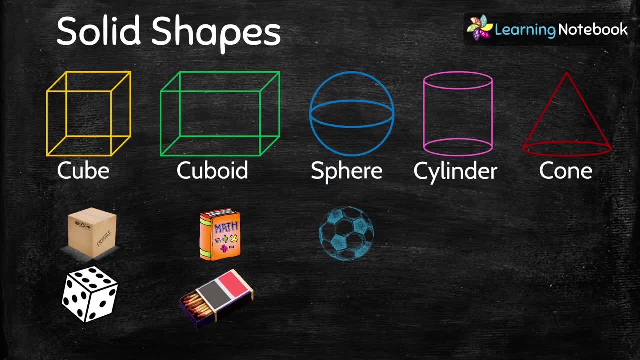 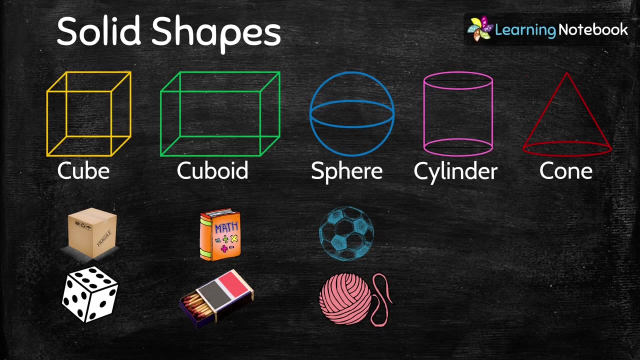 Next let's see examples of sphere, a football and a woollen ball. Students, whenever you kick a football, remember you are kicking a sphere shape. Now examples of cylinder are a pencil and a candle. So whenever you use a pencil, 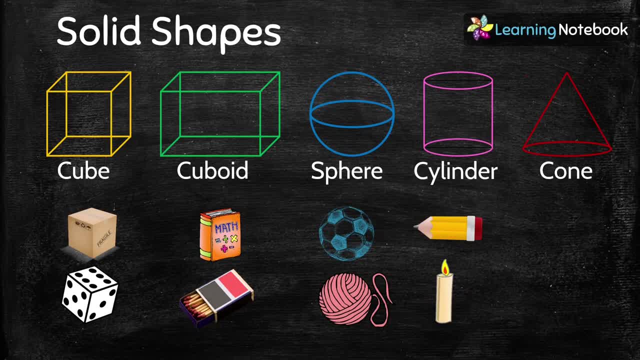 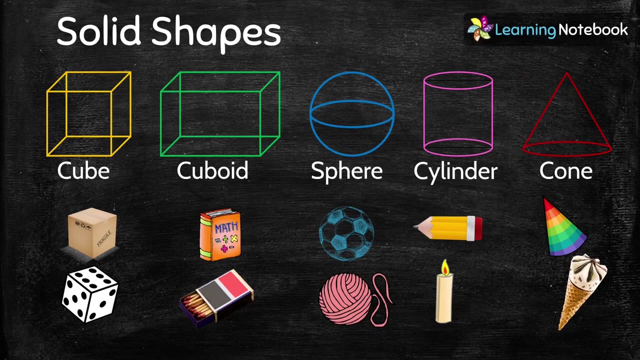 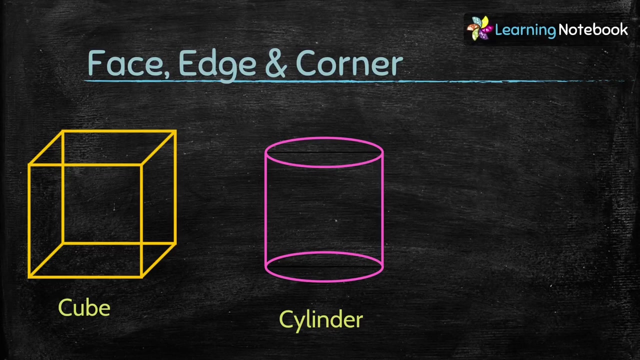 remember it is of cylinder shape. And lastly, examples of cone are a birthday cap and an ice cream cone. So whenever you are enjoying your favourite ice cream cone, remember it is a cone shape. Now let's understand face, edge and corner of a solid shape. 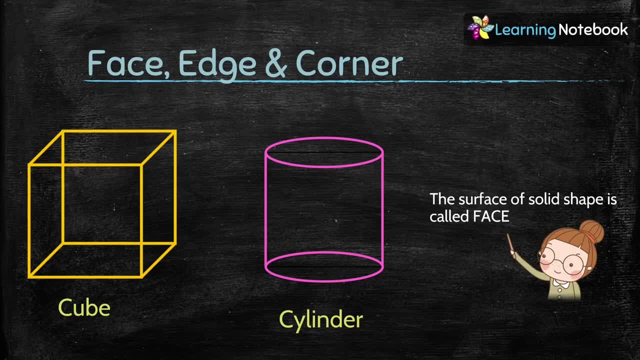 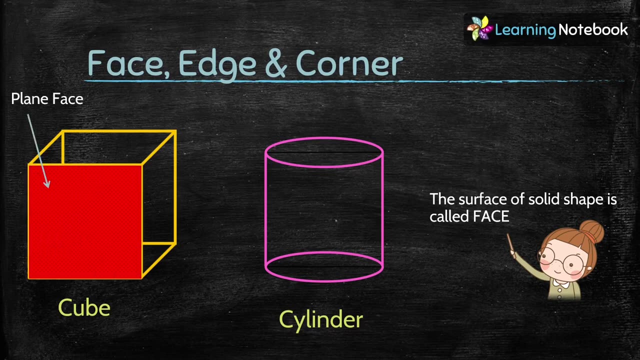 First let's understand face. The surface of a solid shape is called face. As we learnt before, faces are of two types: plain face and curved face, Like in a cube. surface of a cube is a plain face, as shown here. 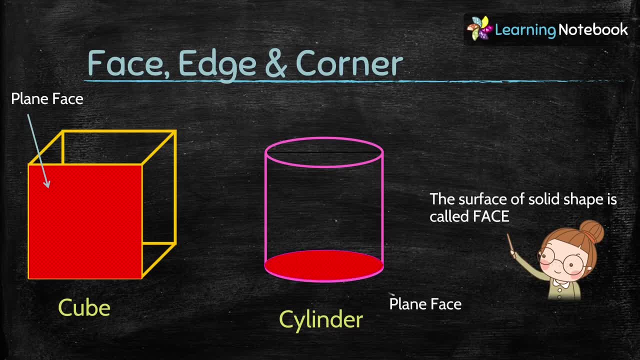 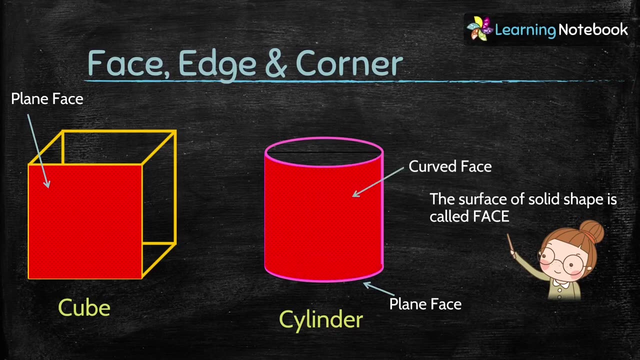 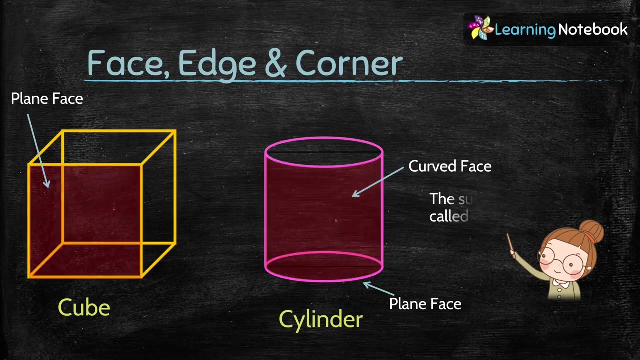 And in case of cylinder, the bottom surface is a plain face, Whereas the curved surface of the cylinder is an example of curved face. So this is the difference between plain face and curved face. Next, let's see what is an edge. 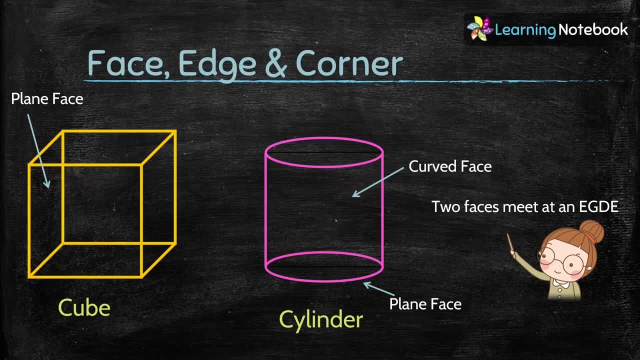 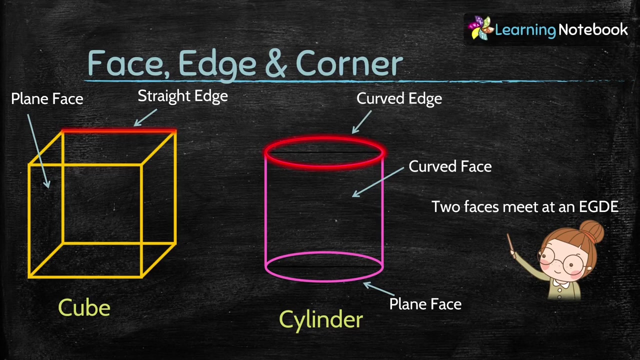 Two faces meet at an edge. Edges are also of two types: straight edge and curved edge. In case of a cube, we only have straight edge, as highlighted here, While in case of cylinder, we only have curved edge, as shown here. 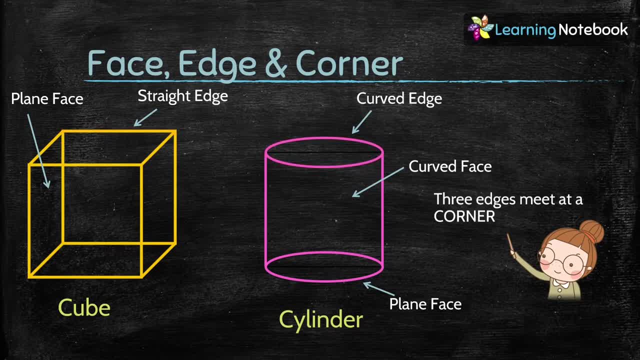 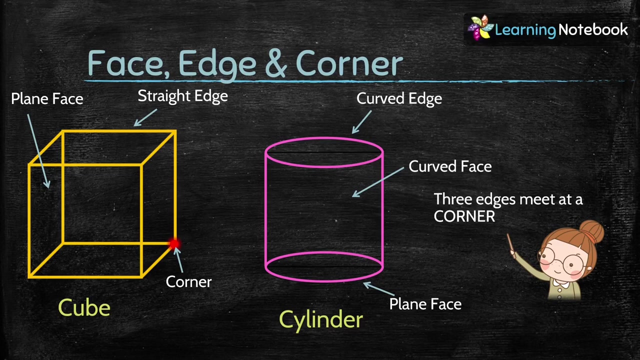 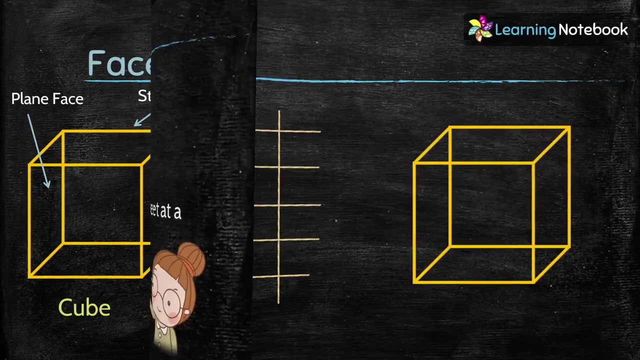 Now, what is a corner? Three edges meet at a corner. Therefore, as you can see in this cube, three edges are meeting at a corner. So this was about face, edge and corner of a solid shape. Now let's take 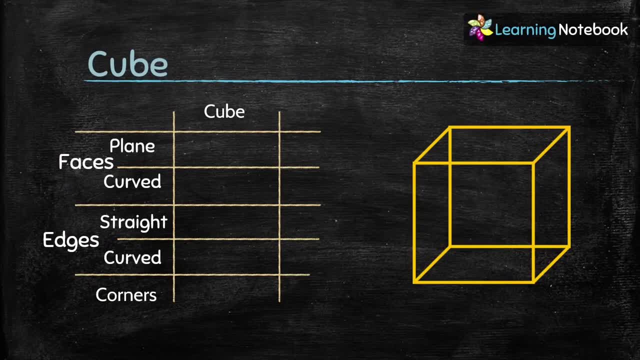 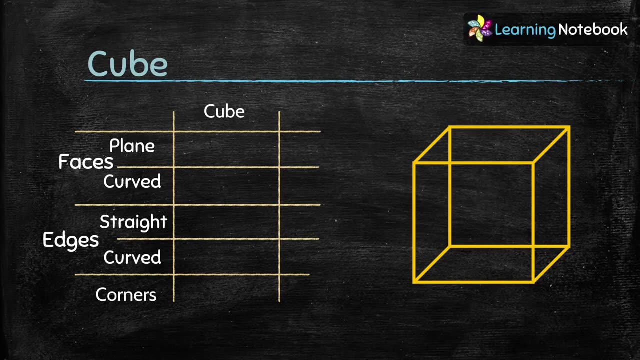 each solid shape one by one And learn about number of faces, edges and corners. First solid shape is cube. A cube has six plain faces. Students, you can easily remember number of plain faces of a cube with the help of a dice. 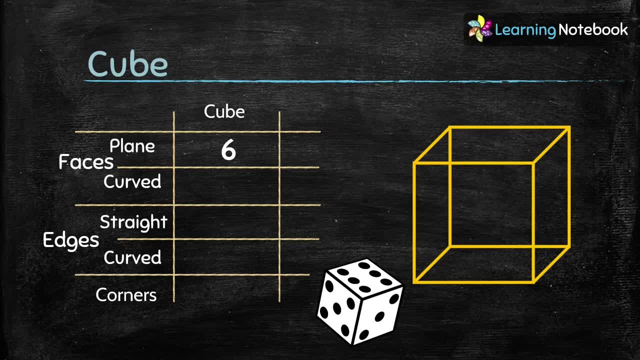 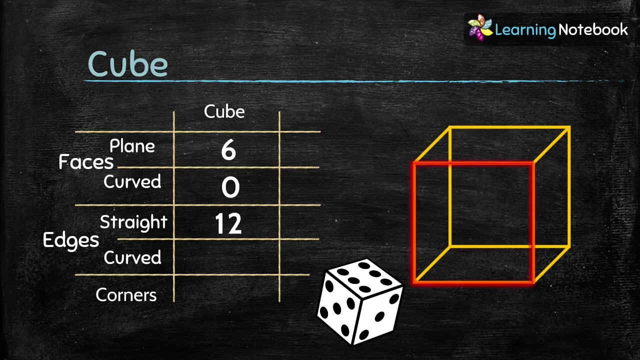 A dice has numbers up to six Because it has six plain faces. Now, curved face: A cube has zero curved face. Next edges, Straight edges. A cube has twelve straight edges: Four on the front face, Four on the back face. 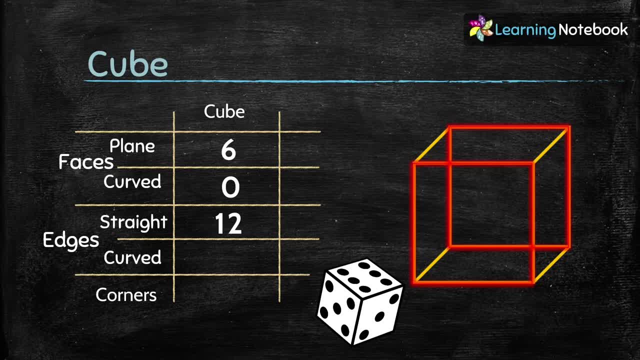 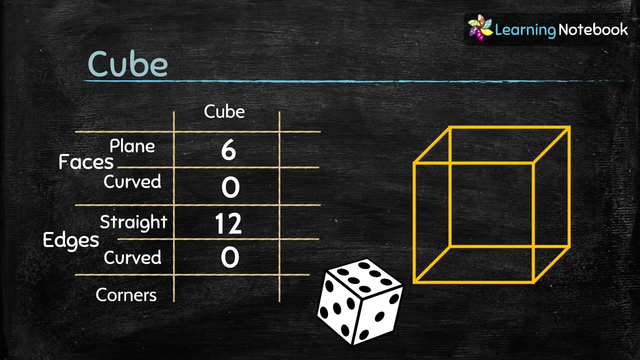 Two on the back face, Two on the top face And two on the bottom face. Now, curved edges: A cube has zero curved edge. And lastly, corners: A cube has eight corners, as highlighted here. Now the next solid shape is: 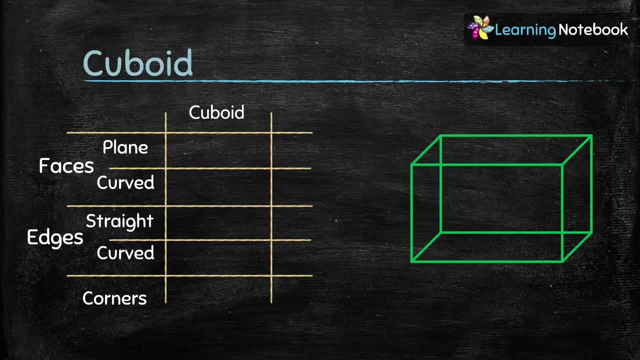 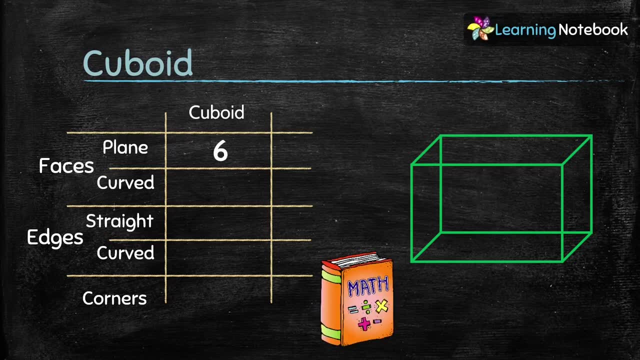 cuboid- Similar to cube. a cuboid has six plain faces and zero curved face Straight edges. A cuboid has twelve straight edges: Four on the front face, Four on the back face, Two on the top face And two on the. 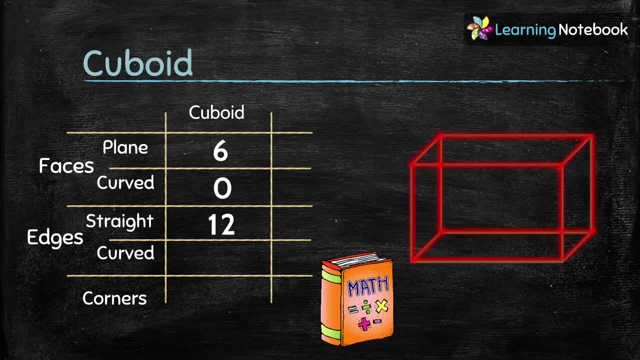 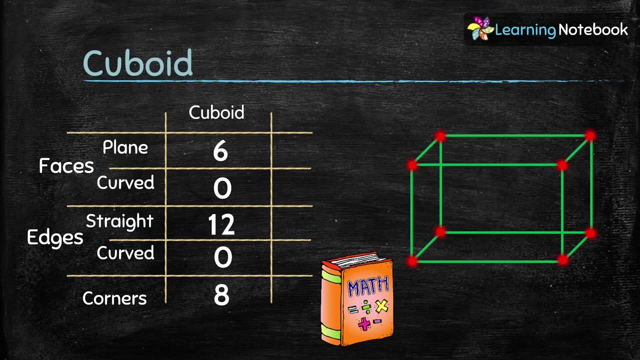 bottom face, And cuboid has zero curved edges. And lastly, corners. A cuboid has eight corners, as shown here. So, students, did you notice? cube and cuboid have same number of faces, edges and corners. Now next is 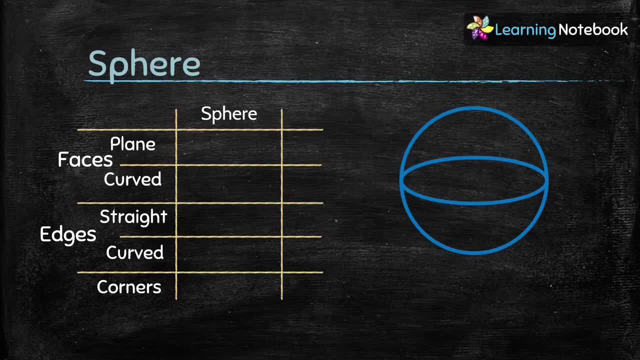 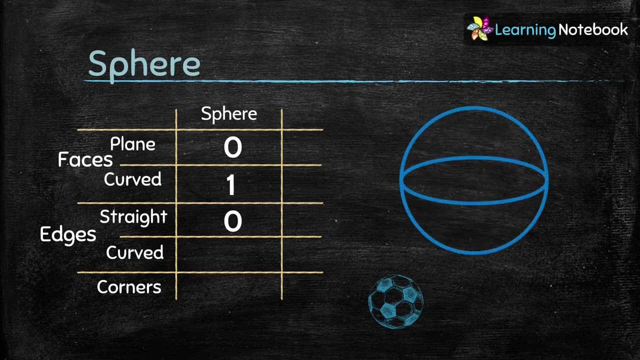 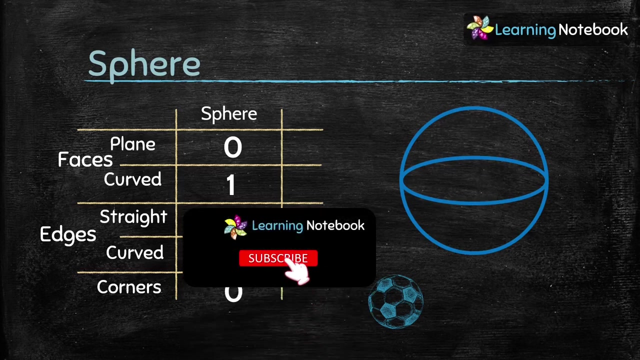 sphere. As you can see, a sphere has no plain face, But it has one curved face. Next, a sphere has no straight and curved edges And, lastly, a sphere has no corners. If you are enjoying watching videos on our channel, then do like. 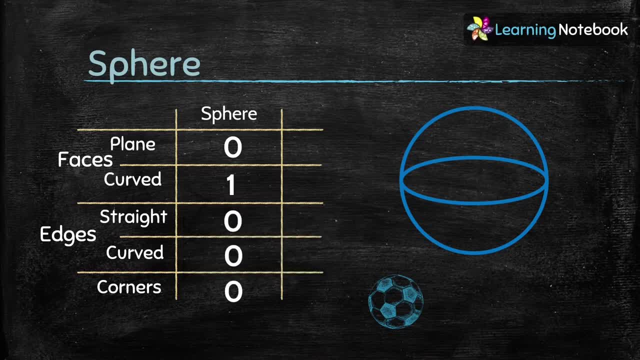 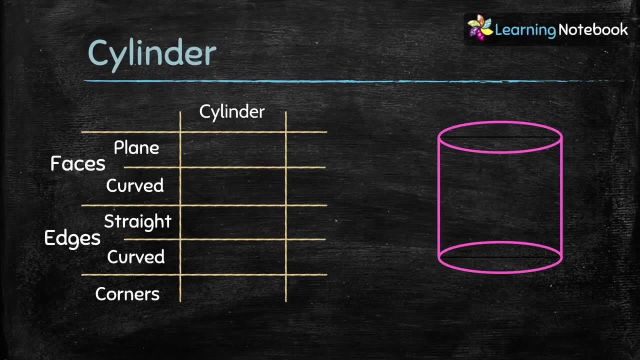 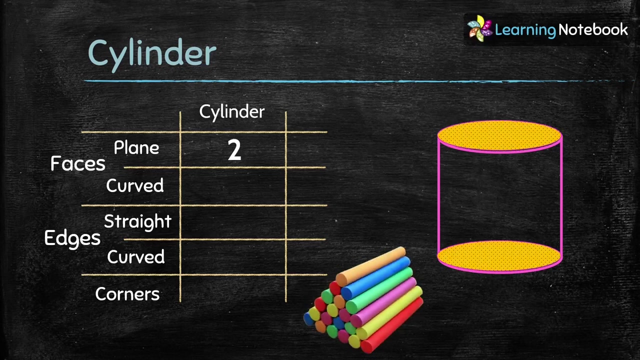 share and comment on our videos. Also, do not forget to subscribe to our channel Learning Notebook. Let's see the next solid shape, which is cylinder. A cylinder has two plain faces, One at the top and one at the bottom, And it has one. 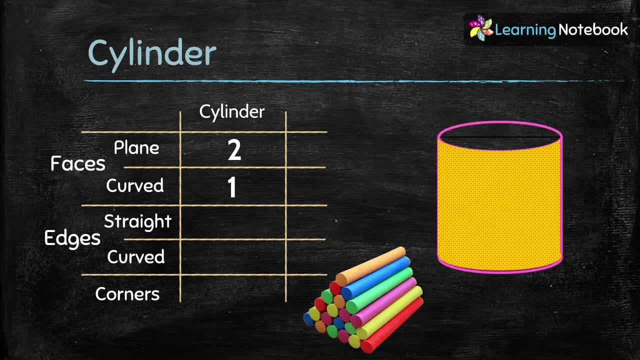 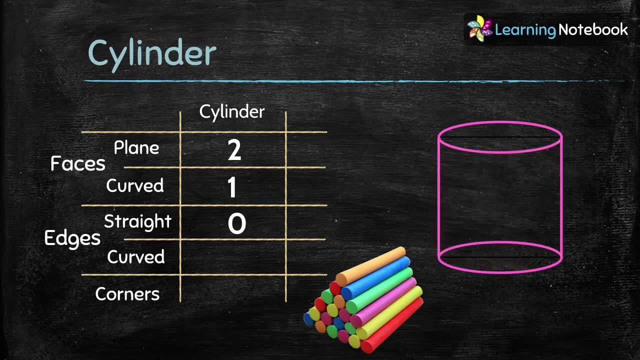 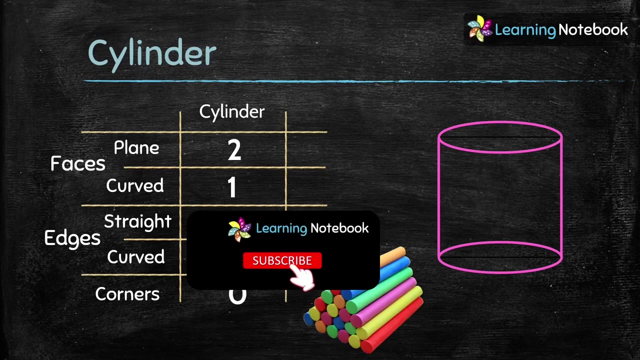 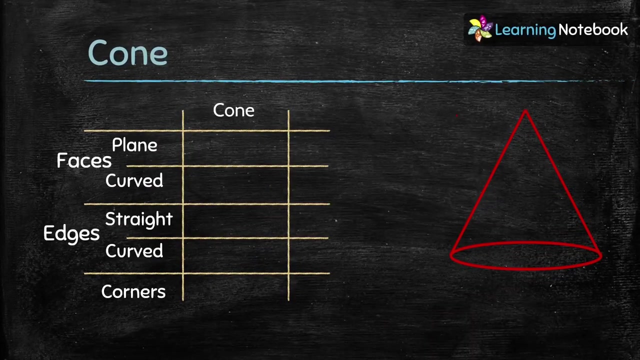 curved face, as shown here. Now edges: A cylinder has no straight edge, but it has two curved edges, One at the top and other at the bottom. And lastly, corners: A cylinder has no corners. Now let's see the last solid shape. 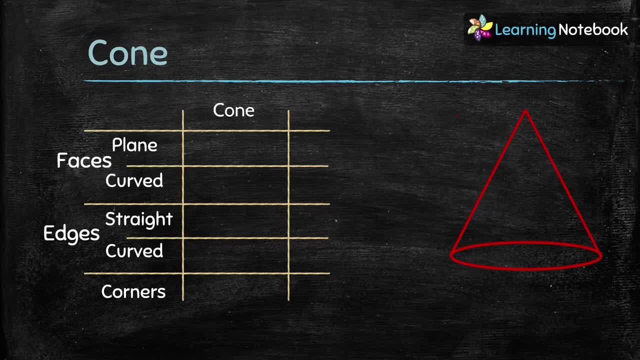 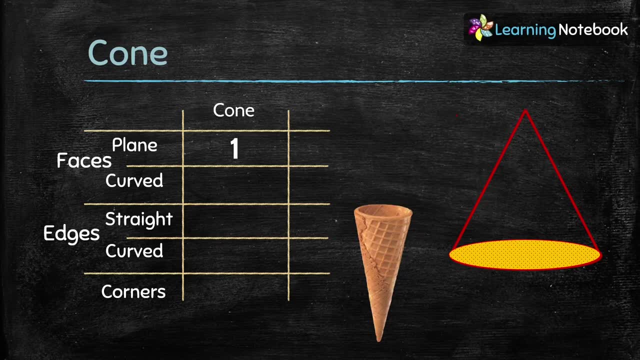 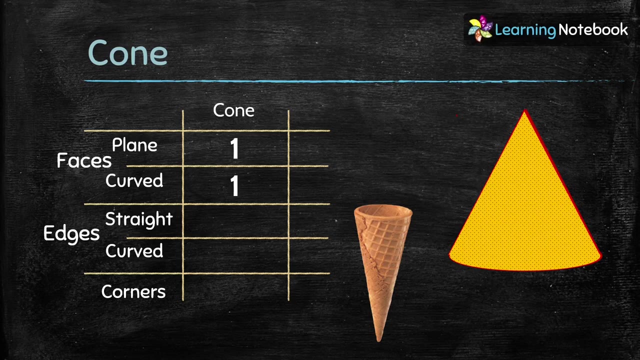 which is cone. A cone has one plain face at the bottom And it also has one curved face, as shown here. Next, edges: A cone has no straight edge, but it has one curved edge. And, lastly, a cone has one corner. 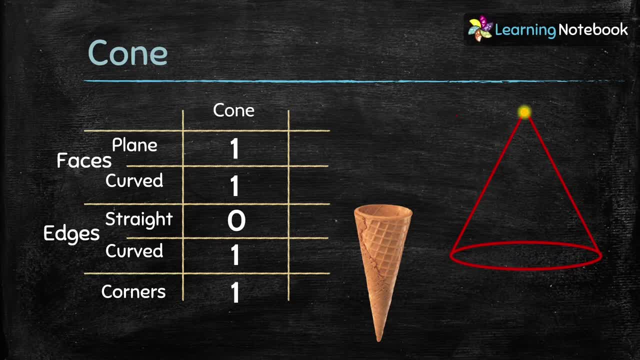 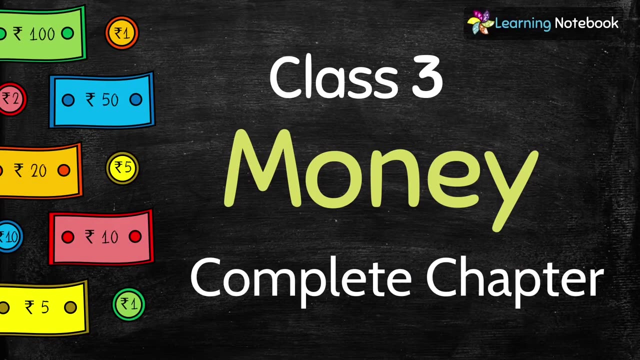 as highlighted here. So, students, this was all about faces, edges and corners of solid shapes. Students, we also have a complete chapter of money for class 3.. Do watch this separate video to understand all the concepts of money. The link to this video is: 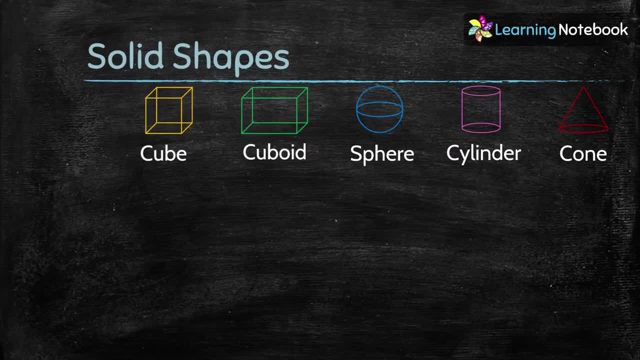 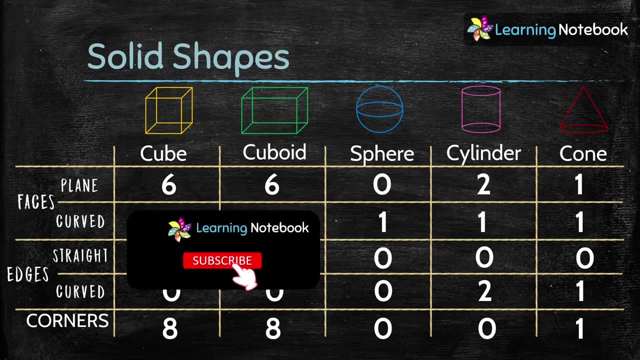 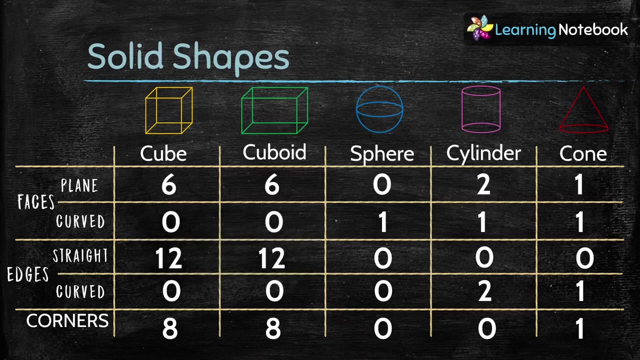 below in the description box. So this is the synopsis of what we learned about faces, edges and corners of 5 solid shapes. Students, it would be really great if you make this table on your own. Then you would be able to remember the number of 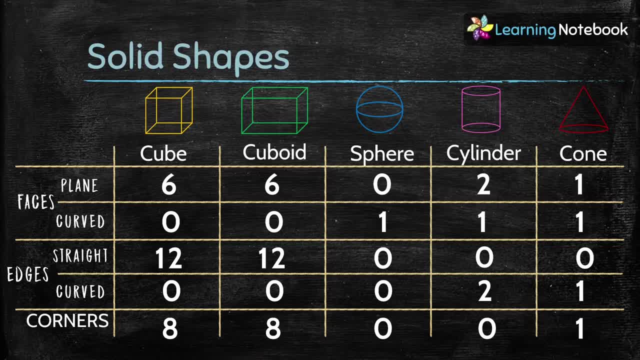 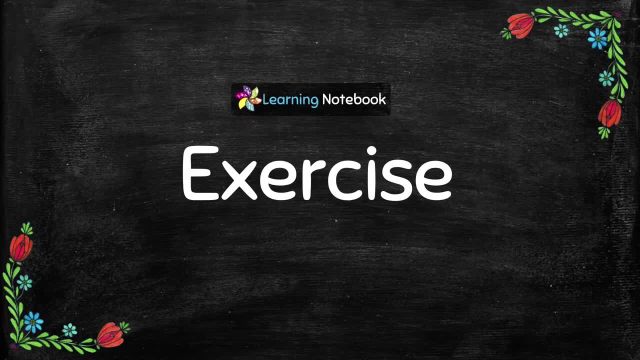 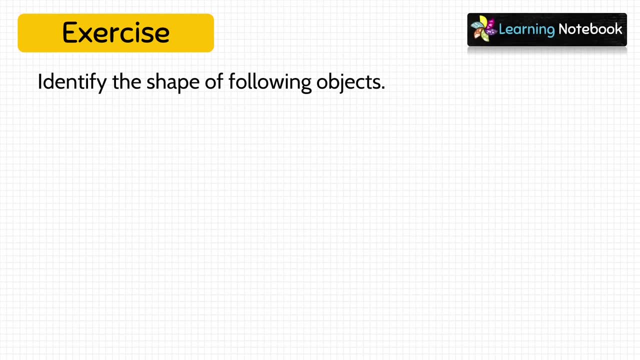 faces the number of edges and corners for each solid shape. Now let's do a small exercise. So question is: identify the shape of the following objects. First is funnel. Can you tell me the shape of a funnel? Yes, it is of cone. 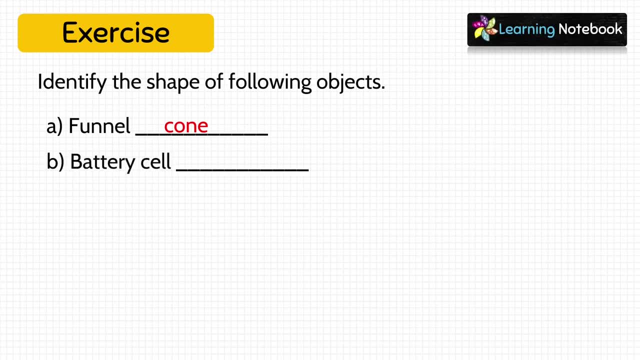 shape. Next, battery cell: It is of cylinder shape. Next watermelon: It's quite easy: Watermelon is of sphere shape. Then we have pencil box. What is the shape of pencil box? Yes, keyboard. And then we have 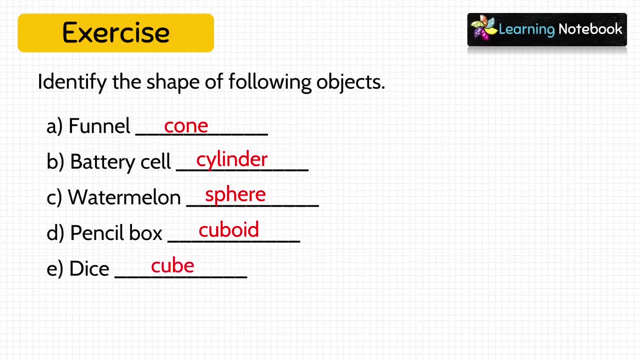 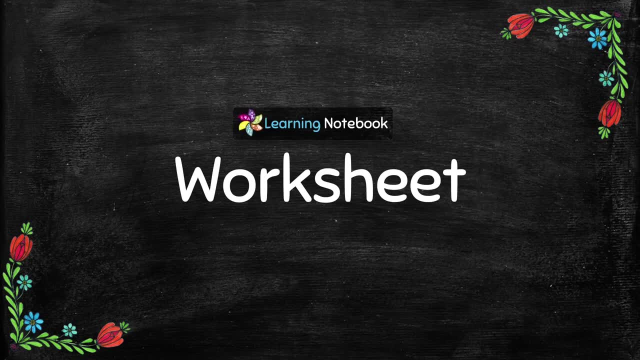 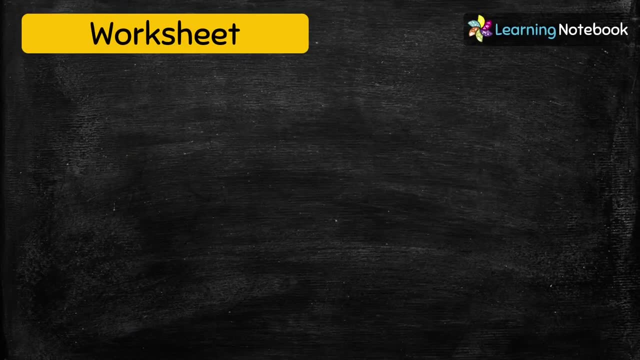 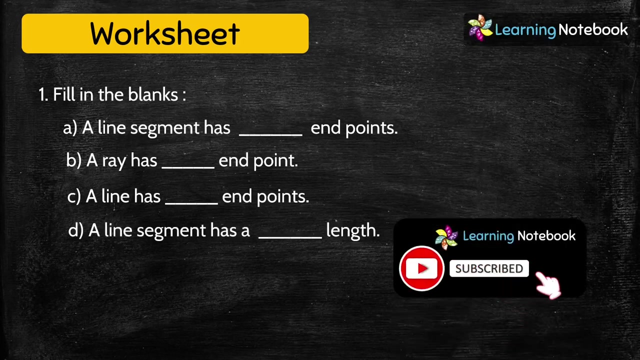 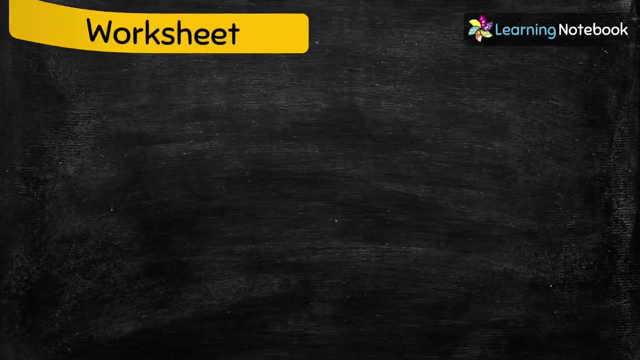 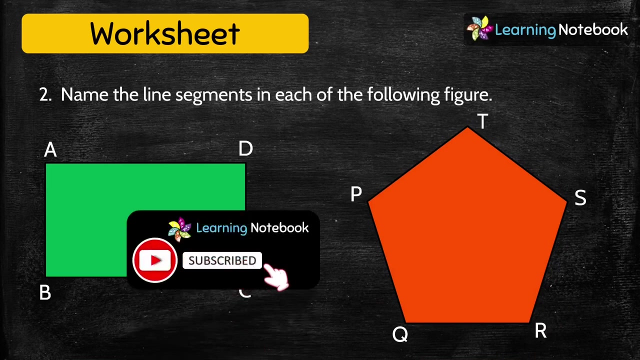 dice. Dice is of cube shape. Now, in the end, I am giving you a worksheet for your practice. This worksheet contains questions from all the sections of the chapter which I have just taught you. If you have skipped any of the section, I will suggest you. 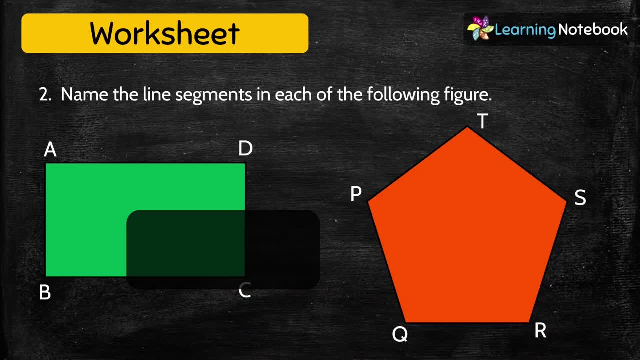 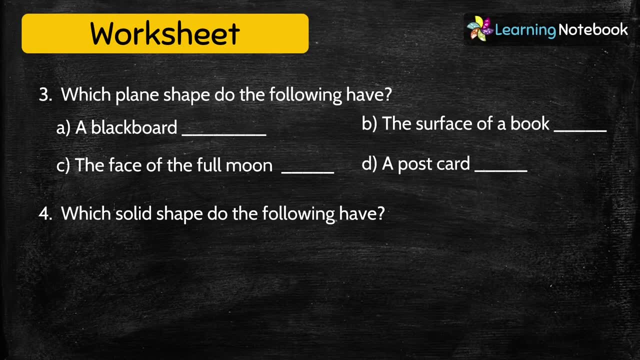 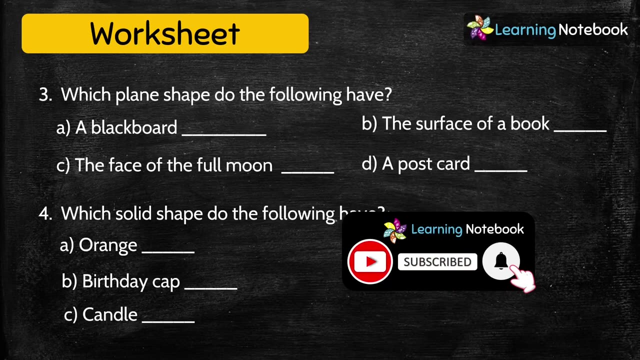 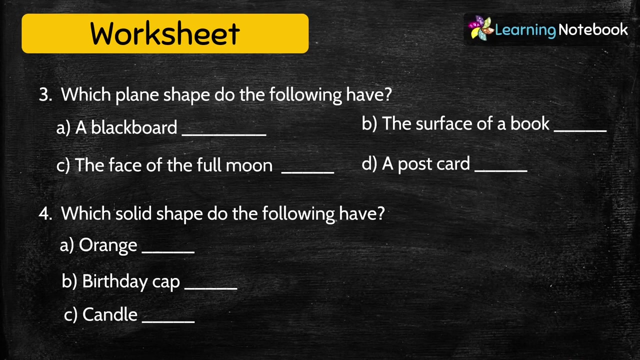 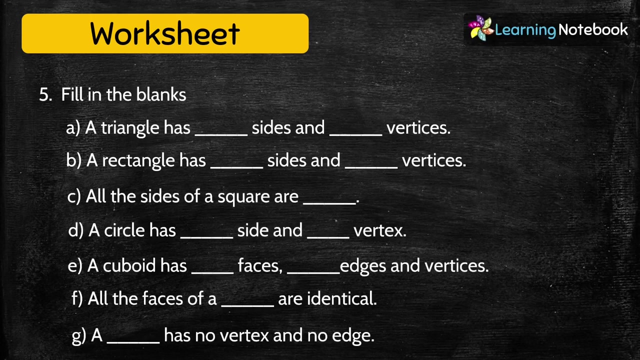 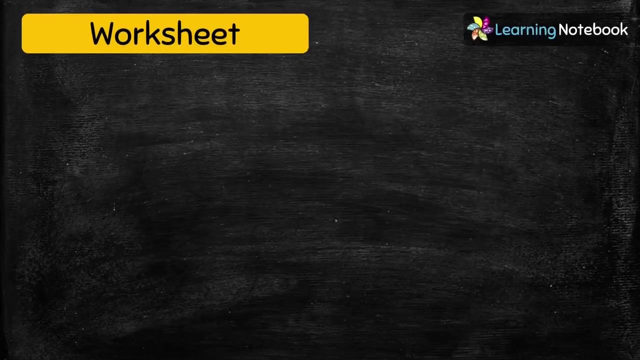 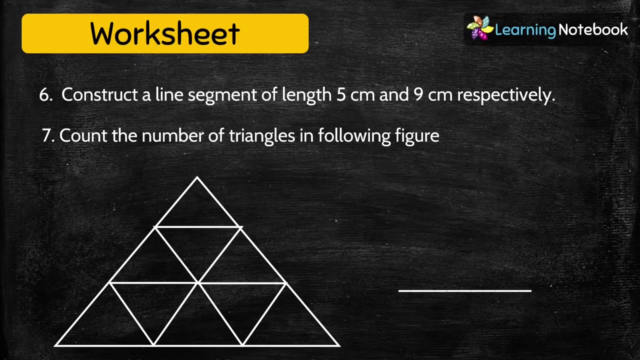 to first understand that section and then attempt this worksheet. Do watch my other videos and share my channel and my videos with your friends and family. Thanks for watching. See you in the next video. Bye-bye.